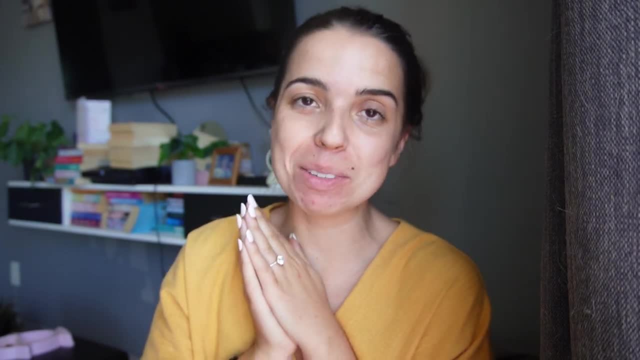 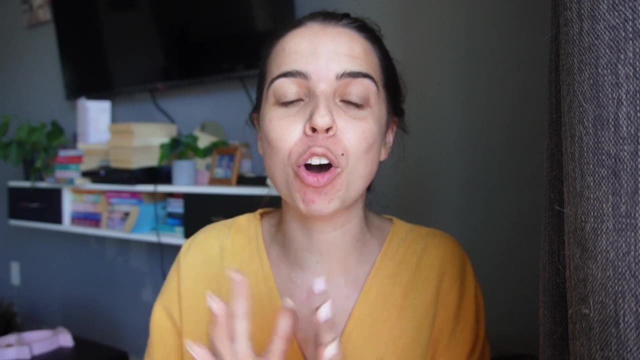 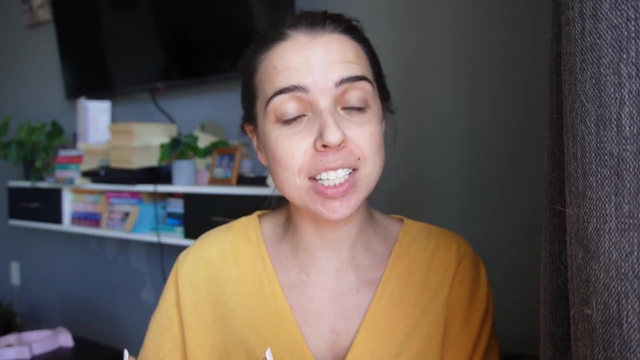 Hello, great tens, and welcome back to another video with me, Miss Martens. In today's video we're going to be looking at electricity, or electric circuits, and this is a summary video of the entire section. Now, with that being said, this is an overview. I don't do a lot of past paper practice in here, but 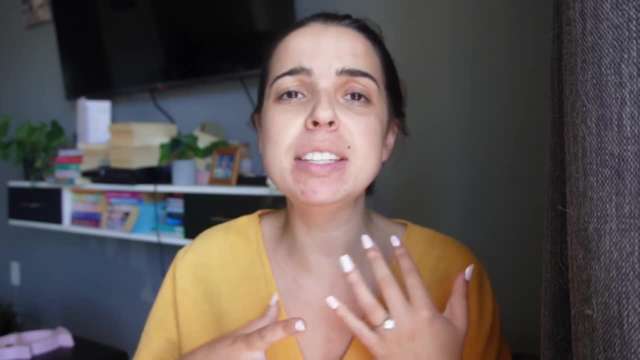 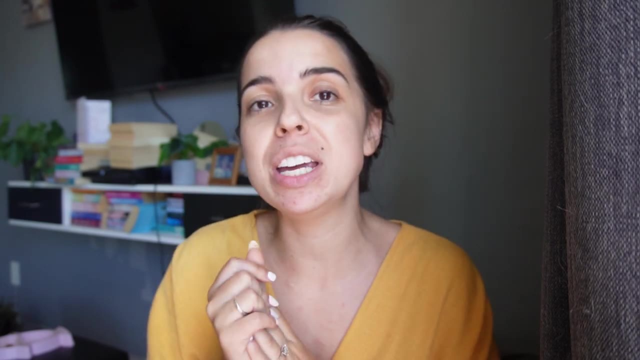 I have that linked in the description box below, But this goes through basically everything that you need to know for your exam. I go through formulas, definitions, concepts, important theory and how to do certain calculations, So I hope that you stick with me throughout the entire video. 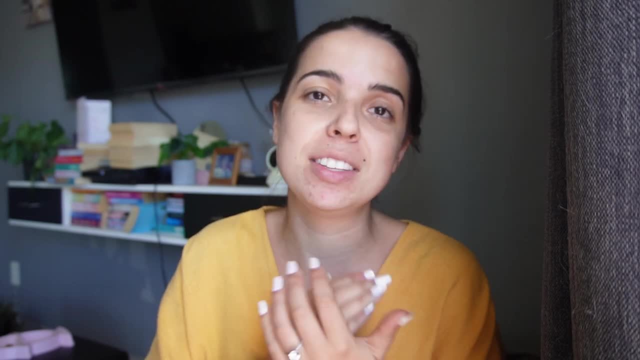 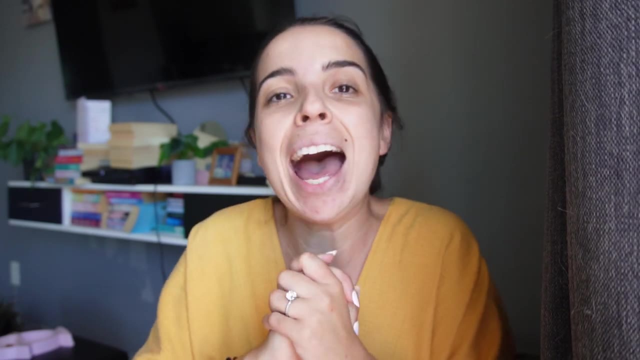 because I give loads of teacher tips along the way. As a teacher that sets marks, moderates exams, I can help you level up your marks. Remember to subscribe for more physics, chemistry and maths. Let's jump right into the video. This is basically an overview of what you need to know for 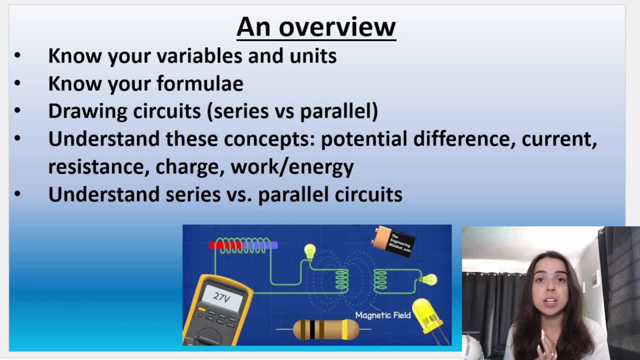 electricity or electric circuits. You need to know your variables and units, know your formulae, know when to use which formulae. You need to be able to draw circuits, both series, parallel resistor connections and a combination of both. You need to understand the listed concepts and you need to understand how to work with series circuits. 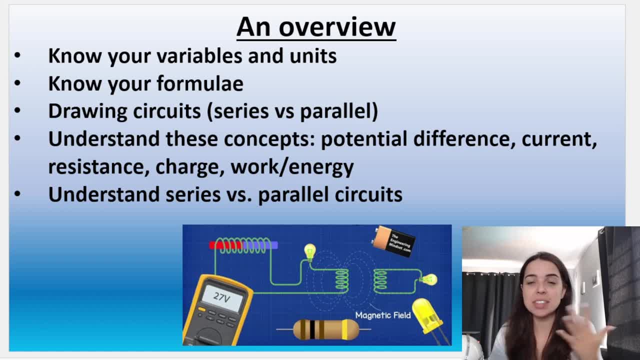 parallel circuits and, once again, a combination of both. So that's what this video is going to be going over. very briefly, Remember it is a summary, so for a more in-depth look at circuits you need to look at the links in the description box below. But you should know that electricity 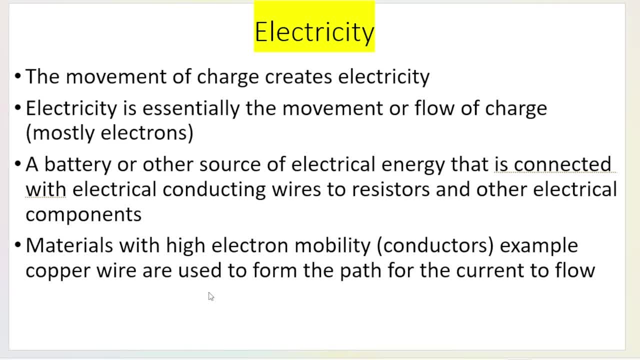 is the movement of charge. The flow of electricity is the movement of charge. The flow of electricity is the movement of electrons and that is what creates electricity. It's the flow of charge, mostly electrons. We have a battery or source of electrical energy that is connected with 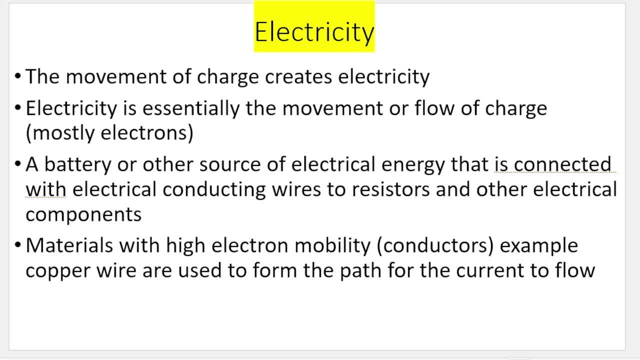 conducting wires like copper wires, resistors or other electrical components. So, for example, we can want to power an appliance, So we can have a battery or a power source connected with conducting wires. We have a light bulb that we want to power. We have a microwave that we want to power. 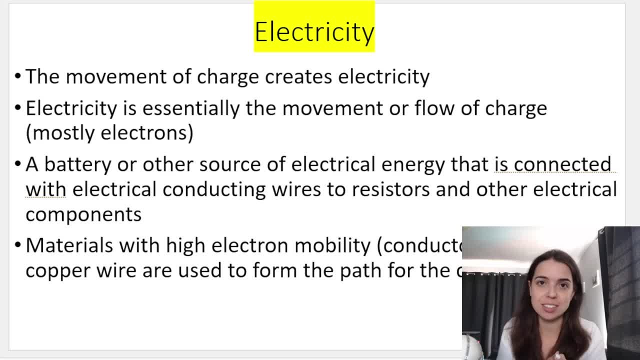 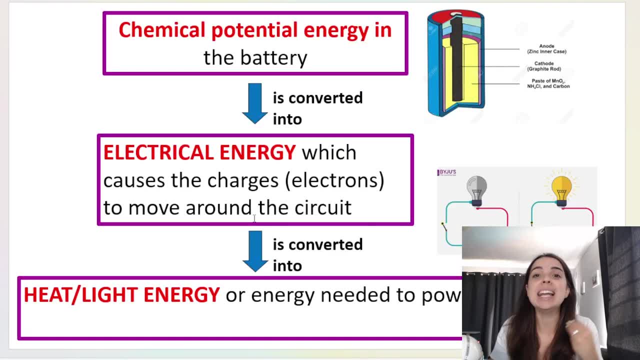 Electricity and this section is all about energy conversion. So we start off with chemical potential energy within the battery and that is converted to electrical energy. So electrical energy is what causes the charges, the electrons, to move around the circuit, and that electrical energy is converted into heat energy or light energy or energy needed to power the appliances. 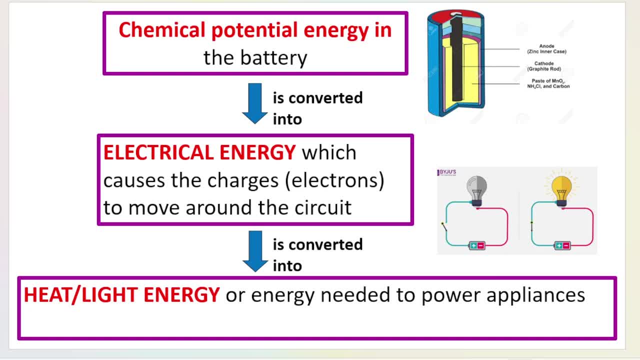 So you need to understand that, So you need to understand that, So you need to understand that This flow of energy and how it's converted or transformed- Remember, energy cannot be created or destroyed, just transformed from one form to another. So this is the flow of energy. It is very 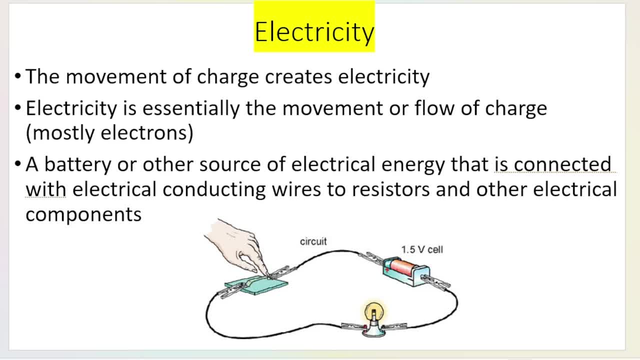 very important to know that we need a closed circuit in order for electric current to flow or in order for our charges to flow, Cannot be an open circuit. Our switch must be closed And you'll often see a discussion surrounding the direction of current flow. 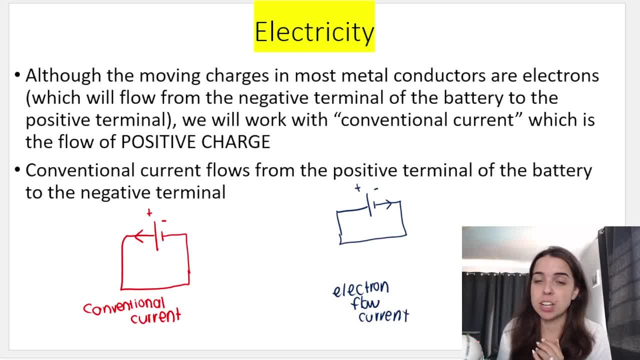 So this says, although moving charges in most metal conductors are electrons, electrons are negative, And think about that. If they're a negative they will flow from the negative terminal of the battery to the positive terminal. That's what makes sense. That's called. 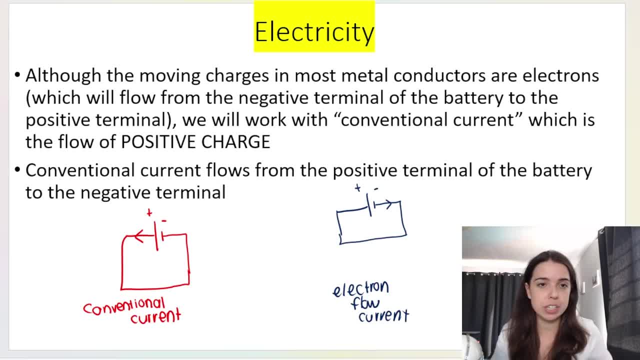 electron flow current. That's the blue circuit I drew over here. So because electrons are negative, they flow from the negative terminal of the battery through to the positive terminal, because negatives are attracted to the positive. That makes sense. It's called a closed circuit. 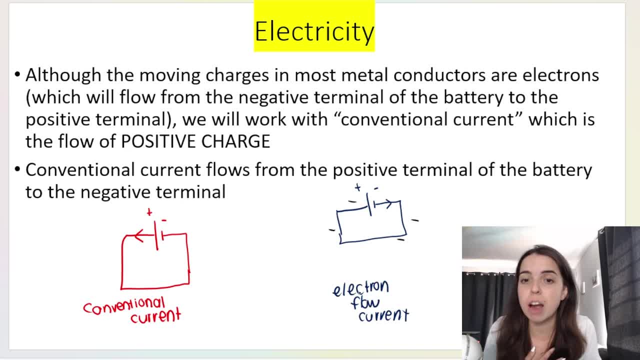 Electron flow current, But we work with conventional current flow, which is current flow from the positive terminal of the battery through to the negative. And just as a reminder, a battery can be represented by the following symbol. like that, The small line is the negative. 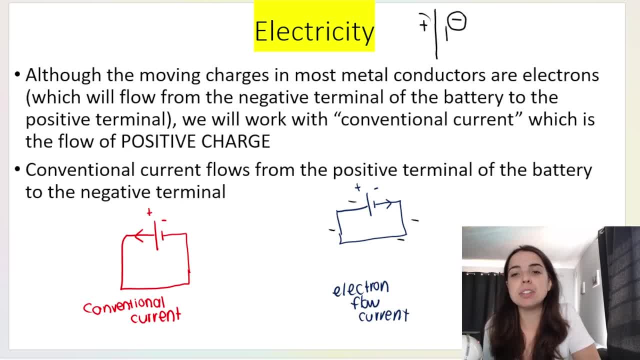 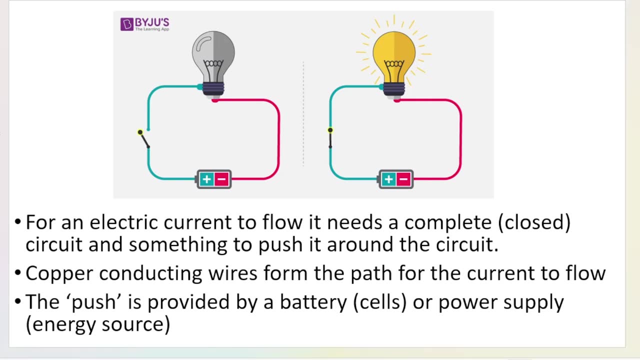 terminal of the battery. The big line is the positive terminal of the battery. So just know the differences between conventional current and electron flow current. We work with conventional current, OK, so, as I mentioned, we need a closed circuit in order for electricity to flow, in order for 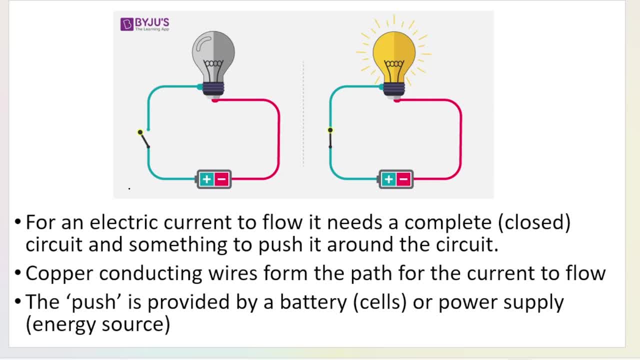 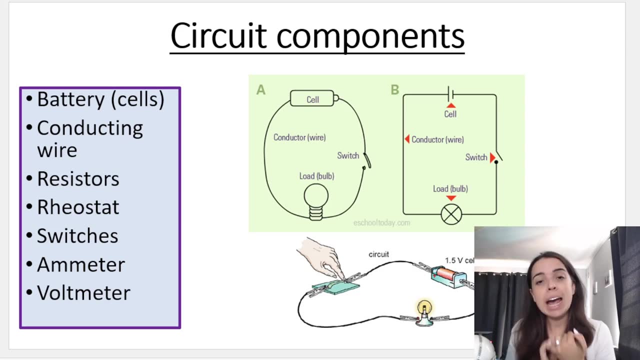 current to flow. The conducting wires, usually copper, provide a pathway for the current to flow and the push comes from the battery. That's my energy source, or my power source. Now, it is very important for you to be able to draw a circuit and to be able to look at a circuit. 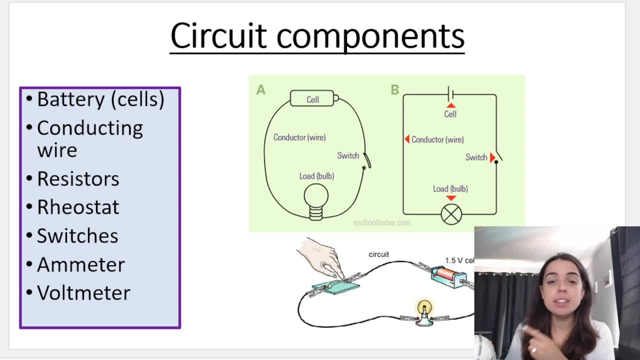 and understand what the different components are. So I've listed some components that are important for you to be able to draw a circuit and to be able to look at a circuit. So I've listed some components that you will be seeing in circuits And it is important to understand. 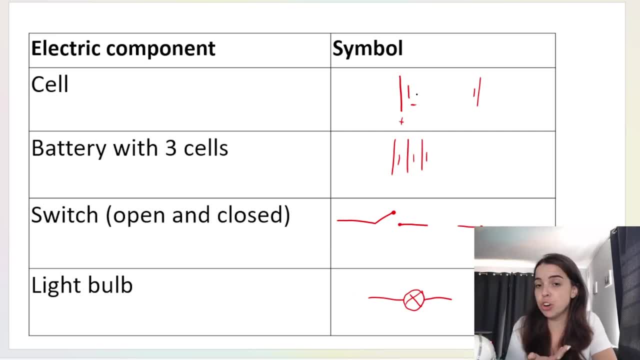 the symbols. So a cell looks like this, As I've shown you: the long line is positive, The small line is negative. This is representative of a battery with three cells. So what they could say to you is that the voltage across the battery is six volts And if I have three cells, that means 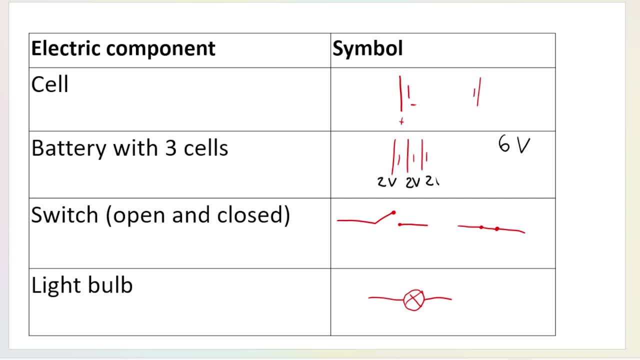 that each battery will have an EMF of two volts or each cell, Sorry. So two volts, two volts, two volts together it gives me six volts. You need to understand that this is an open switch and a closed switch. Remember, switch must be closed in order for the current to flow and the circuit. 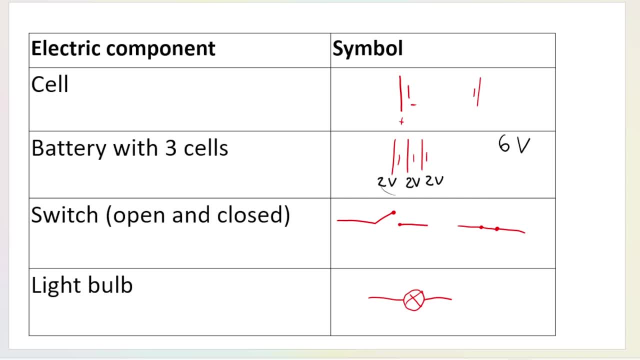 to function. This is how we draw a light bulb. There are more than one ways. There's more than one ways often to represent light bulb or resistor. This is generally what we use. So a light bulb looks like that, a circle with a cross in it. Then we've got a normal resistor. You will either see. 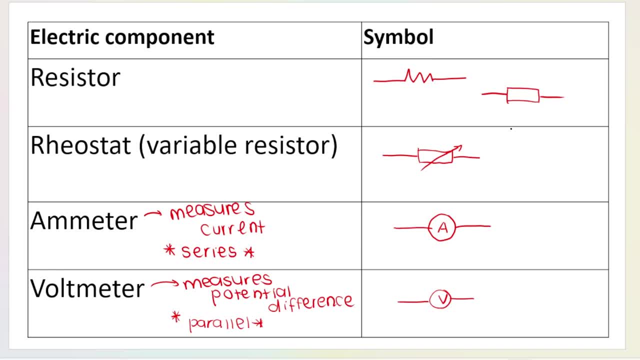 a resistor represented with a circle or a cross in it, And then we've got a normal resistor Squiggly line like that, But more commonly in our curriculum it looks like this, like a little box: Okay, That's a resistor. A rheostat is a variable resistor, So we can change the resistance. 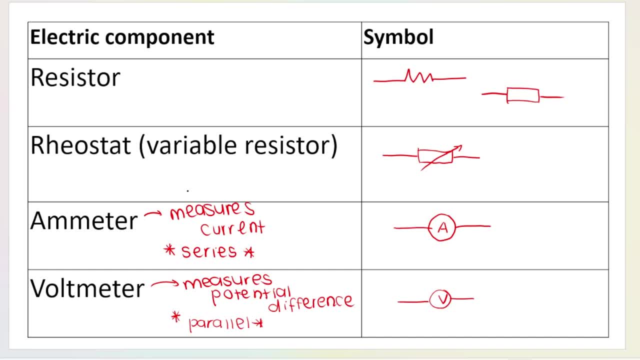 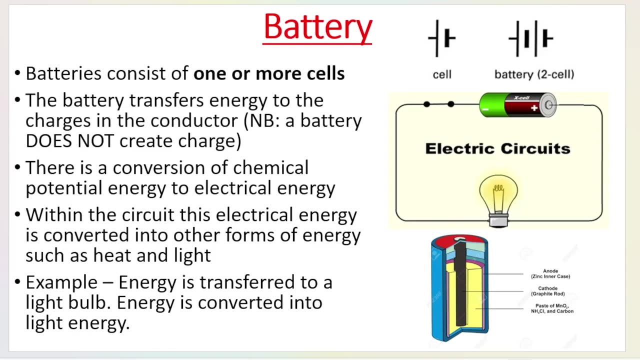 of a rheostat. An ammeter measures current and it's always connected in series. A voltmeter measures potential difference or voltage, and it is always connected in parallel. I will show you what that means in a second. This basically just. 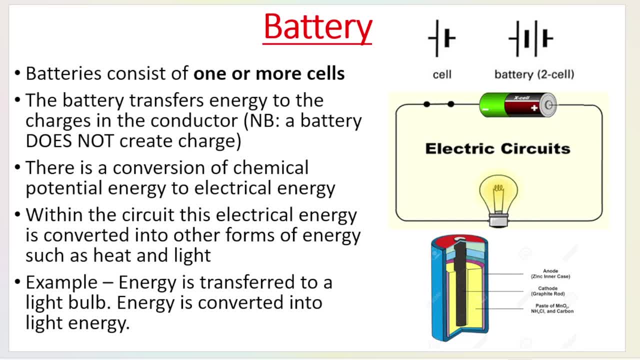 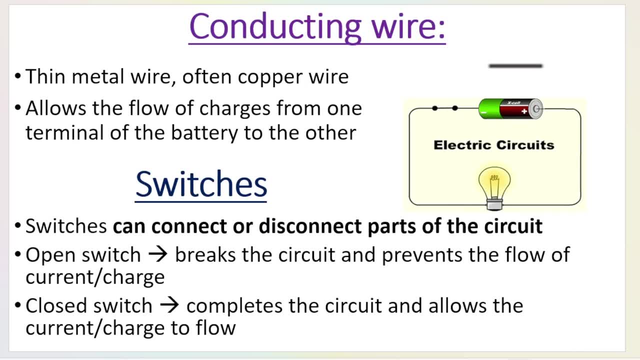 goes through the different components. So a battery consists of multiple cells. I speak here about the energy conversions which we've already been through. Conducting wires are metal wires, often copper, and they attach to the terminals of the battery. They allow the flow. 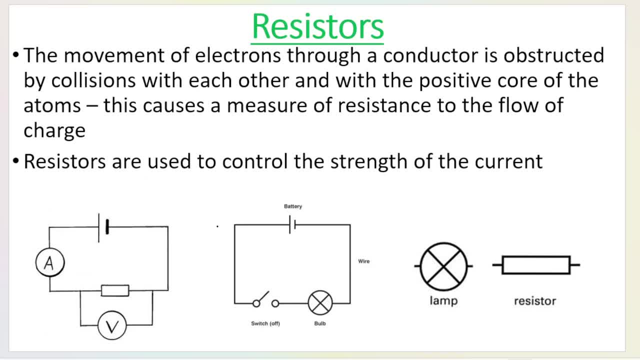 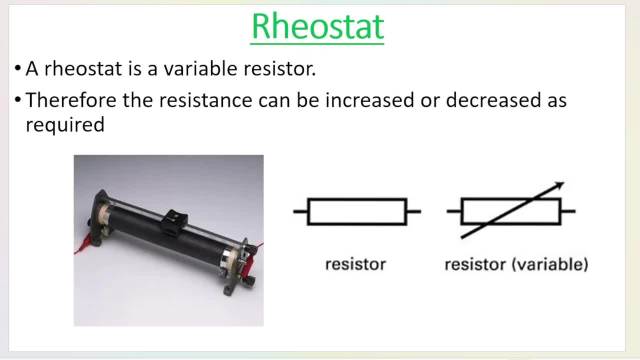 of current. Then they speak about resistors. So this is a resistor. A light bulb is also technically a resistor- a light bulb or a lamp. We've got rheostats, as mentioned. It has an arrow through it to show that it's a rheostat. 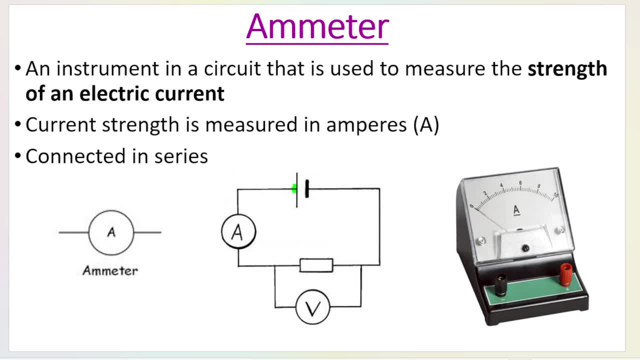 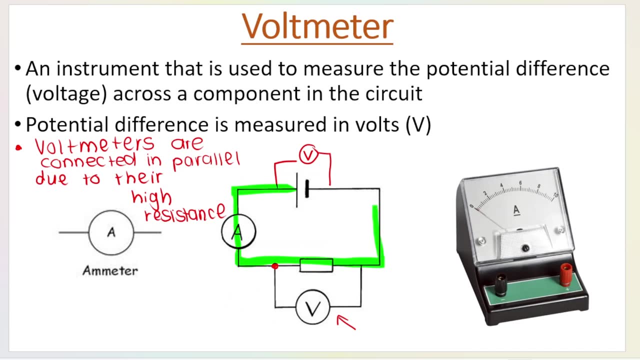 The ammeter is connected in series. So here we can see this is the main line of the circuit. The ammeter is connected in series, So it's connected along the main line of the circuit. You can see that a voltmeter is different. Here's the main line of the circuit. There's the main line of the circuit. 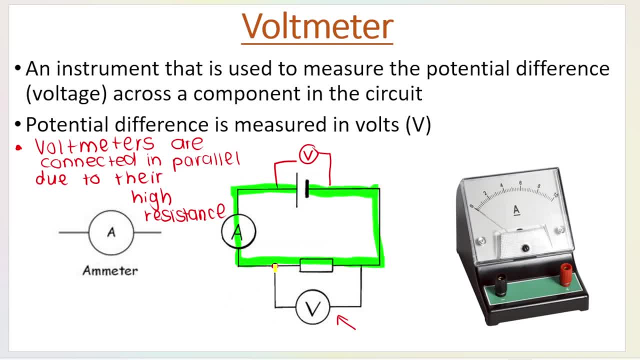 The total current flows through that main line, The voltmeter branches off, which means it is connected in parallel. And the reason why voltmeters are connected in parallel is because they have a very, very, very high resistance, which means that current does not. 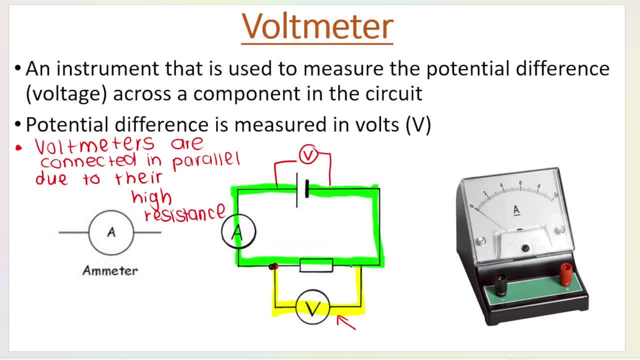 want to flow through them. What this means is that if I decided to connect the voltmeter in series like this- so if pretend that instead of the ammeter we have a voltmeter- If I had to connect a voltmeter in series, the total resistance of the circuit would be way too high, which means 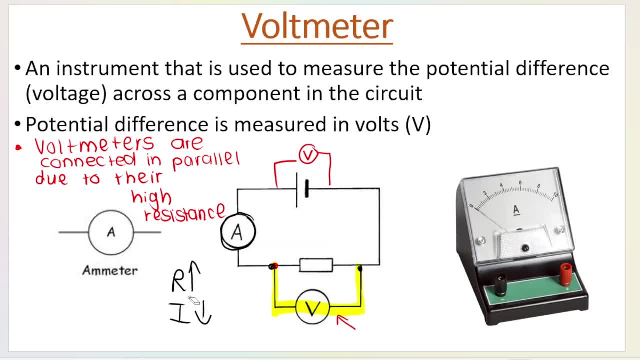 current would be tiny and the circuit would not function, So I'm going to connect it in parallel like this, because the current does not want to flow through here. All that this voltmeter does is it measures the potential difference between two points in a. 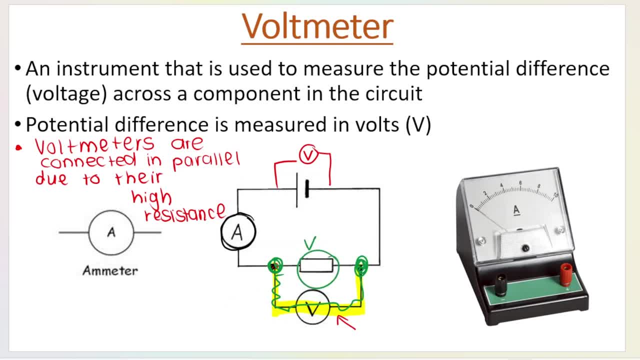 circuit. So, for example, it tells me the voltage or the potential difference across this resistor, or this voltmeter over here would tell me the potential difference or voltage across the battery. The current does not want to flow through there. Right Now, before I show you the 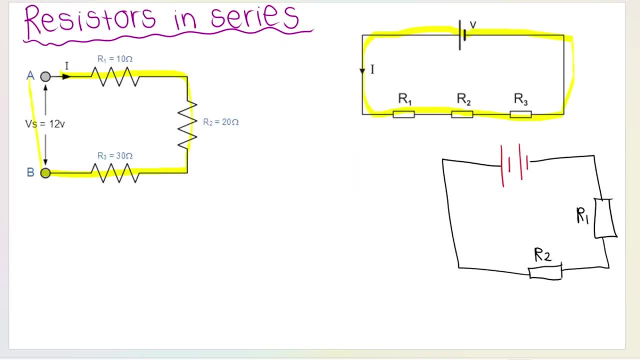 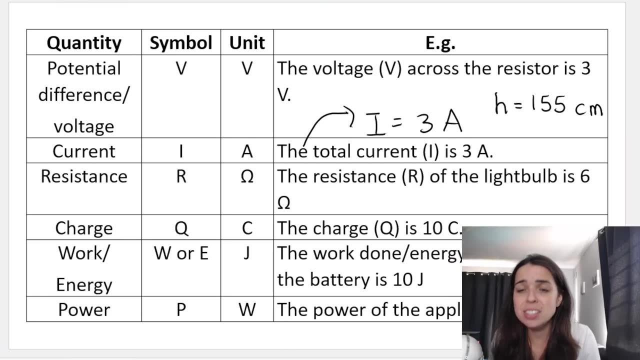 difference between resistors connected in parallel and series. I want to go over the different variables within an electric circuit and grade 10s, 11s and 12s. This is so, so, so important. I mark papers all the way up to metric level and I often see that students get confused. 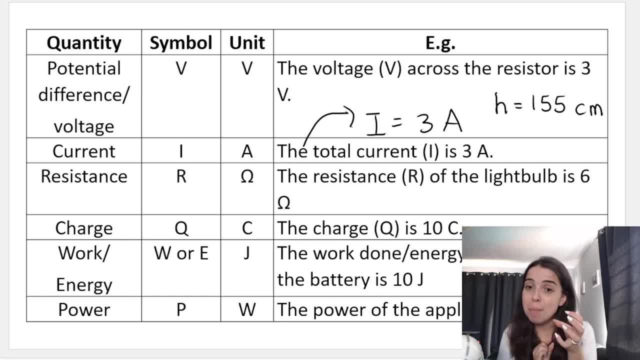 between the quantity- okay- and the symbol to represent that quantity and the unit, There's a massive, massive difference. So I've made a table summarizing what that difference is. I've listed all the different quantities that you will see. I've listed all the different quantities that you will see. 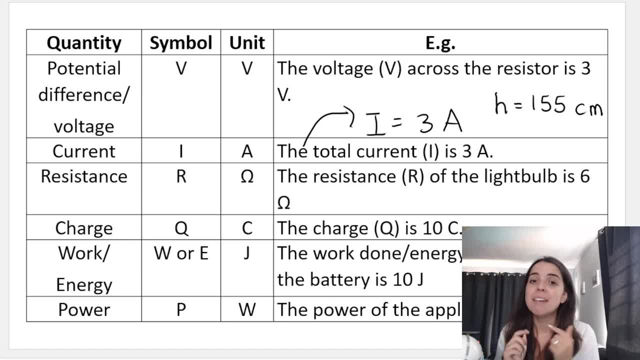 Throughout electricity or electric circuits, the symbol and the unit, and I've given an example of how we use it. So, starting from the top of the table, we've got potential difference or voltage. The symbol for that is V and the unit for that is V. So, for example, if I want to say the potential, 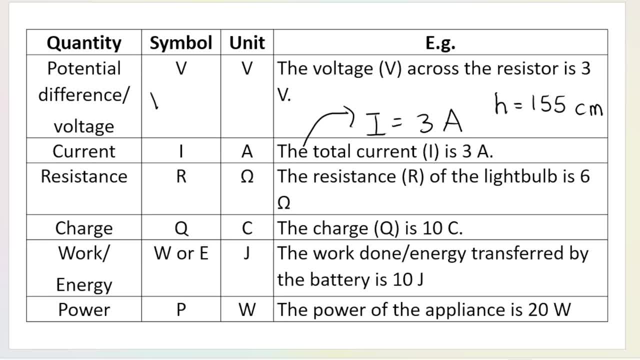 difference across the battery is 10 volts, I say the potential difference across the battery is equal to 10 volts. This is the symbol. It's basically a placeholder. instead of writing potential difference or instead of writing voltage. okay, I explain it over here, like if I say my height is 155 centimeters, instead of writing 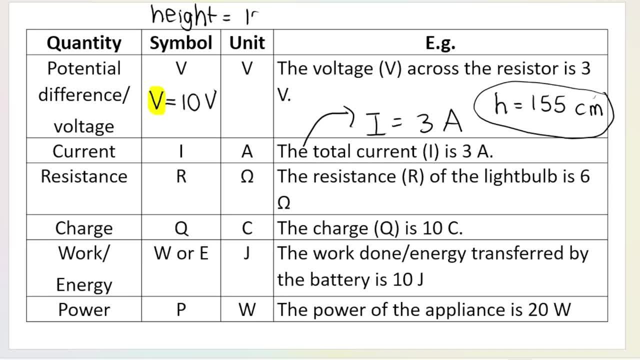 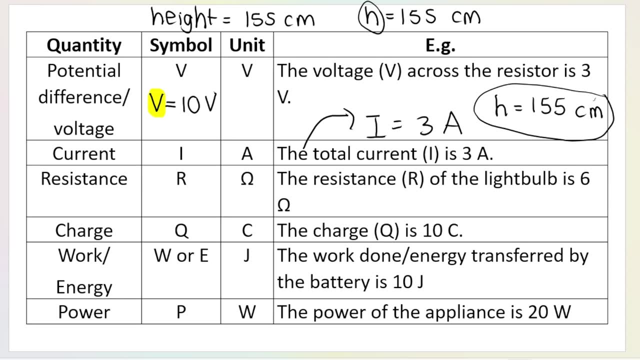 my height is 155 centimeters, I can say H is equal to 155 centimeters, So H is a symbol. It's like a shortened version of writing out height. the unit is centimeters. okay, so the unit always comes after your answer. it is very, very very. 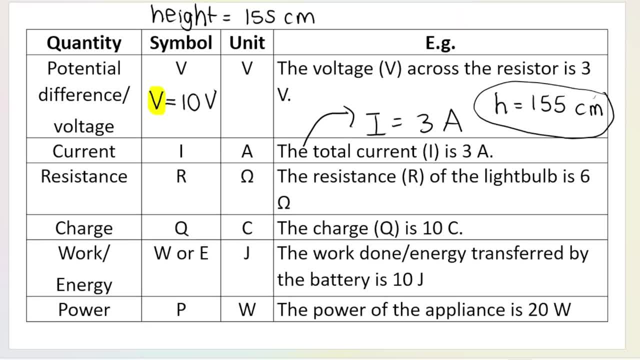 different to the symbol and learners often get this confused in the context of current. so if i want to say the current, the total current in the circuit is three amperes. instead of writing, current is equal to three amperes. amperes is the unit. instead of writing, the current is equal to three. 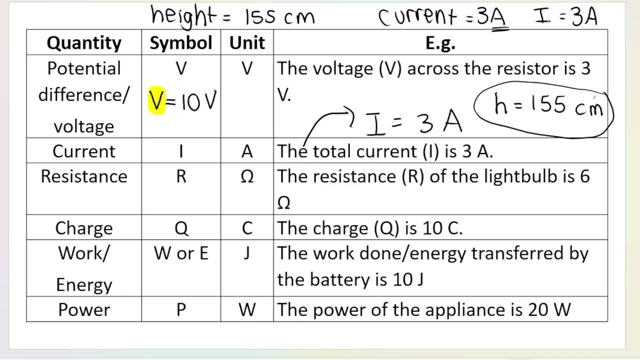 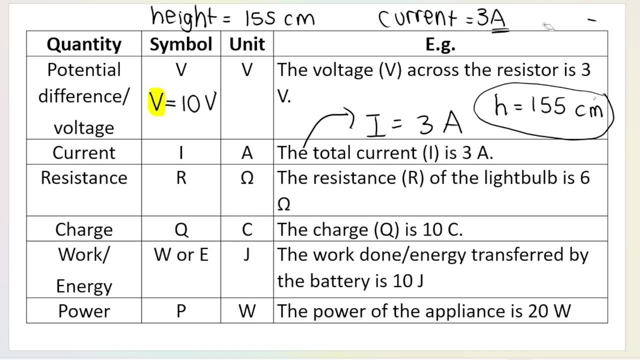 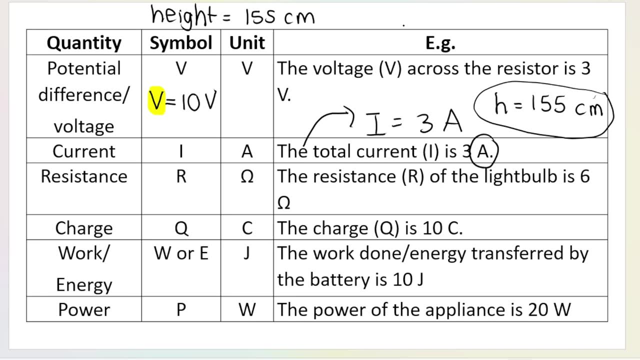 i can write. i is equal to three amperes. i is a symbol for current. okay, cool. now, while i'm speaking about symbols and units and stuff like that, it is very important to note that you must write a as your unit for current, not amps. i know some teachers, some textbooks, some youtube videos. 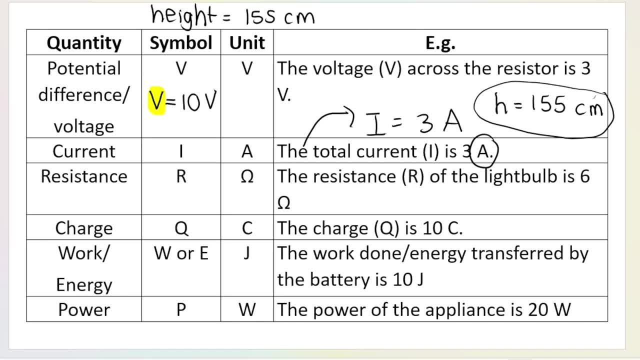 may informally refer to a as being amps. that's incorrect. we actually mark that wrong. so if you say three amps, we're going to take away your answer mark because amps is an incorrect unit. you either write a or you write out the full word amperes. i know that that might sound silly. 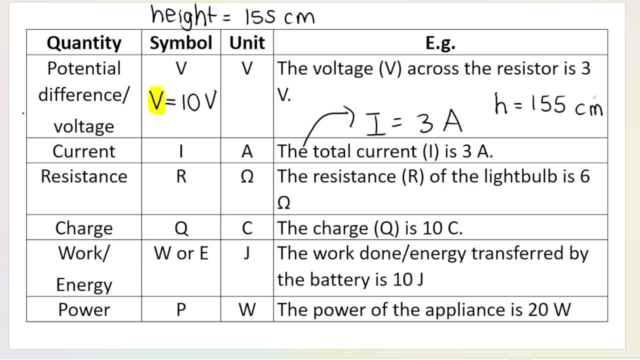 um, but and a little bit pedantic, but that is how we mark. okay, then we've got. resistance is measured in ohms. that's the symbol for ohms. you say ohms charge, the symbol is q and it's measured in coulombs. c is coulombs, the charge is 10 coulombs. work or energy, they mean the same thing. so work done. 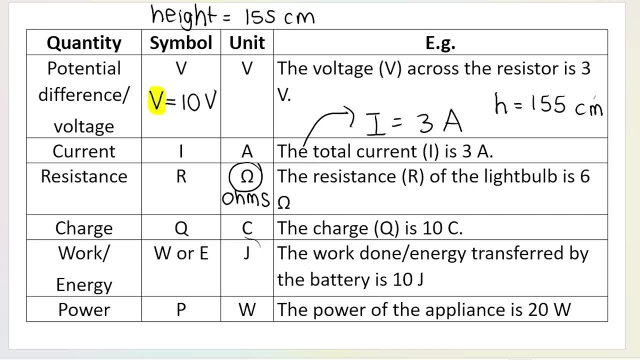 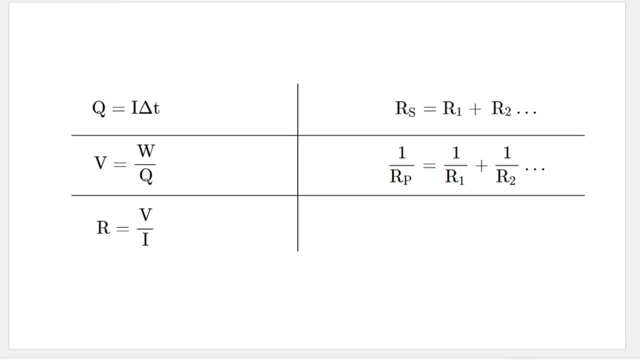 or energy transferred is measured in joule j power p is measured in watt, watt. okay, those are my symbols for my quantities and those are my units. it's very important to know those. then, in grade 10, this is the formula sheet that you receive in your exams. 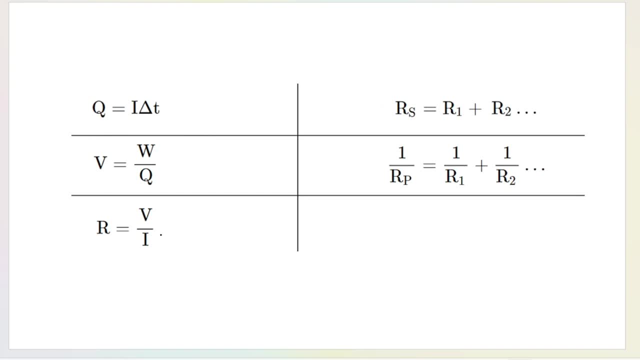 now in grade 11 and in grade 12, you add, we add a lot more formulas, especially those relating to work or energy and relating to power. however, these are my basic formulae and you need to know this whether you're in grade 10, 11 or grade 12.. so let's quickly go over what these 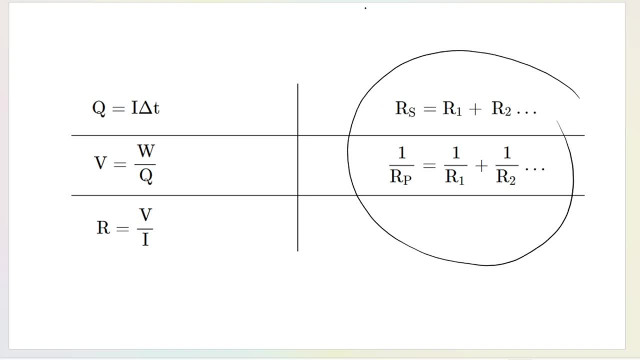 formulas are. these formulas are to calculate resistance within a circuit. if my resistors are connected in series, i use this formula: r1 plus r2 plus whatever. if i have three resistors, then my formula needs to include r1, r2 and r3. if i have two resistors in series. 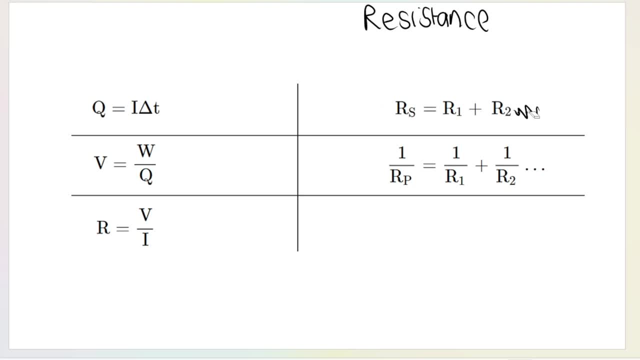 my formula will stop over there. i hope that makes sense. this is for series resistors. then if resistors are connected in parallel, which i will go over in a little bit- in this video we use one of rp is, one of r1 plus one of r2. if i just have two resistors in parallel, you stop over there. you. 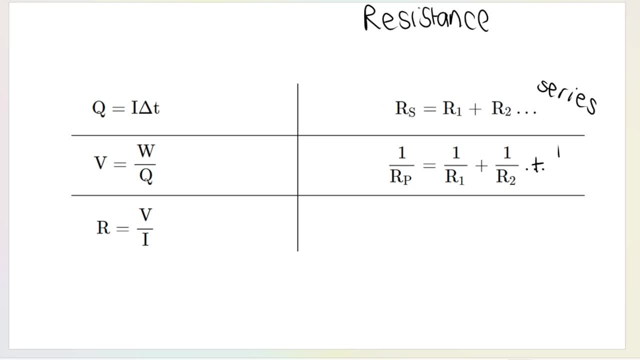 don't have to put the dots. if i have three resistors in parallel, it goes one over r3. so those are my formulas in order to calculate resistance, and remember resistance is measured in ohms. this formula over here is used in order to calculate charge. okay, so the amount of charge. 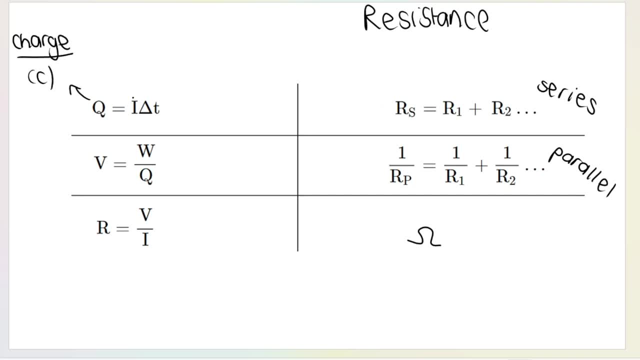 transferred in a circuit, charge is measured in coulombs, or we can use this formula to help us calculate current. remember, current is measured in amperes and then this is time, and this is very important to note. but in this formula, time must be measured in seconds. it's often given in minutes. we need to convert. this formula is used to calculate. 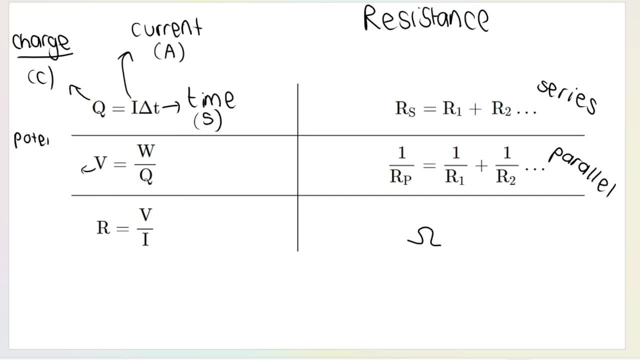 potential difference or voltage, very, very important. please take note that potential difference and voltage, it means the same thing. i know we often refer to it as voltage, you know informally. but potential difference is a more correct term. it's measured in volts. w is work done or energy transferred. remember, although the formula says w. 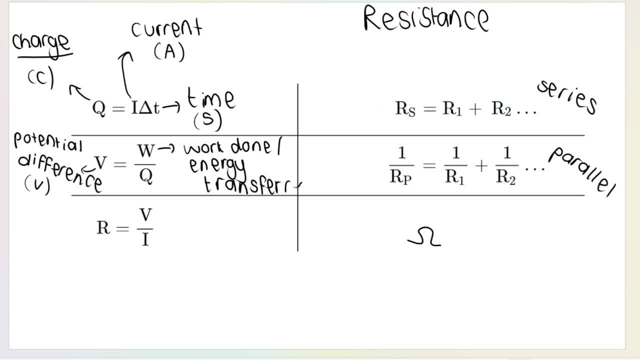 as in work, work done. they can also give it to you in terms of energy. work and energy are the same thing. it's measured in jewels. we spoke about q. q is charge, measured in coulombs. this formula over here is representative of what we call ohm's law. you may see it represented in a. 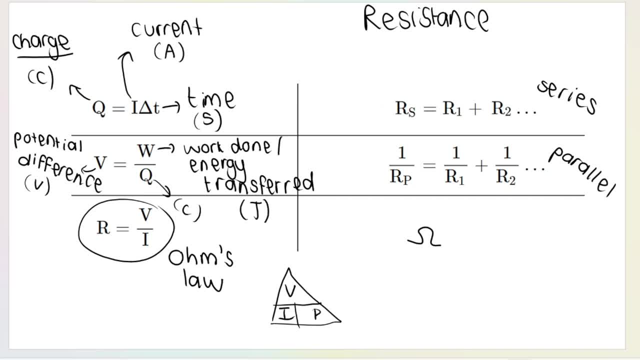 triangle like this: v, i, r, r is obviously resistance. it's measured in ohms, v is potential difference or voltage measured in volts, and i is current measured in amperes. you need to know when to use which formula and in order to know that, you need to understand your quantities or your variables. 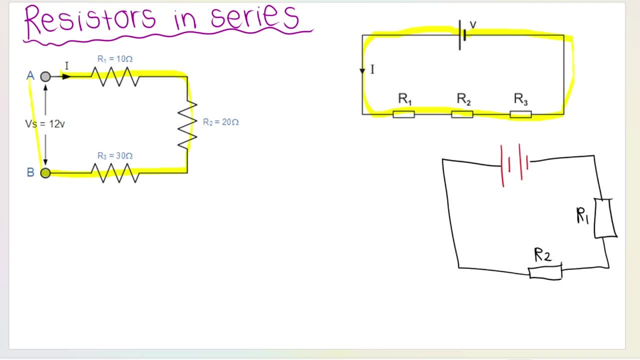 a massive part of completing electricity and circuit questions is knowing and being able to recognize when our circuits and our resistors or components are connected in series, versus when they are connected in parallel or when there's a combination going on. so resistors and series. i have highlighted this already, but i'll show you once more. 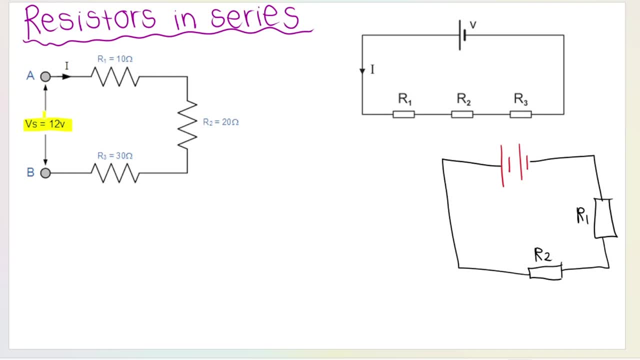 if i start by the battery- and this is supposed to be a battery- and i follow the main line of the circuit. so you take your highlights or you take your finger and you follow the main line of the circuit. like this, you can see that r1, r2 and r3 are all connected in the same line, the main line. 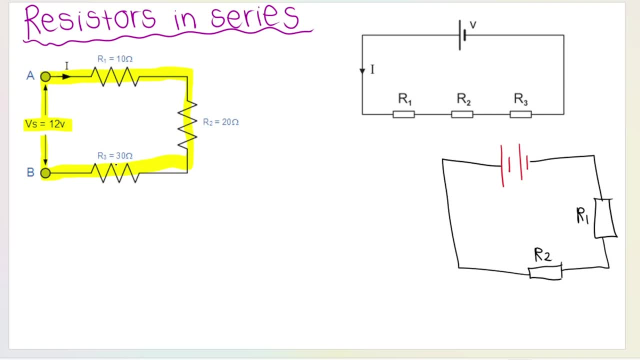 of the circuit. there are no branches, which means r1, r2 and r3 are connected in series. in order to calculate the total resistance of the circuit, you will say r1 plus r2 plus r3. you will simply add them up: 10 plus 20 plus 50, and that is equal to 60 ohms. that's how you calculate resistance resistance. 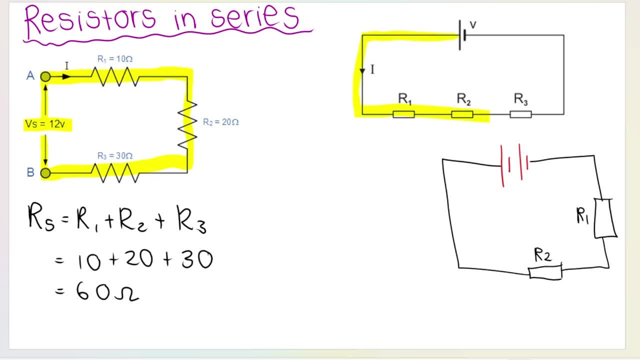 in series. super easy. same thing with this circuit: they're all connected in series. and same thing with this circuit over here: they're both connected in series. as you can see, it doesn't matter if i draw r1 and r2 next to each other or r1 and r2 both connected into series, based on how thenet and 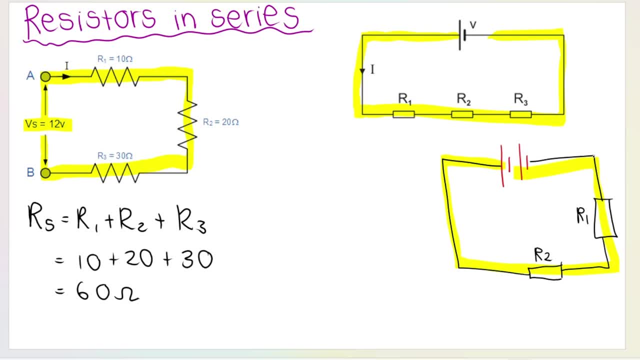 output K were connected to each other, we're able to calculate the present 줄 in the sentence so and to compute the present pleased. that isZA revolution, which means you are all connected to each other. R1 over here and R2 over here, they're still in the main line of the circuit. therefore they are 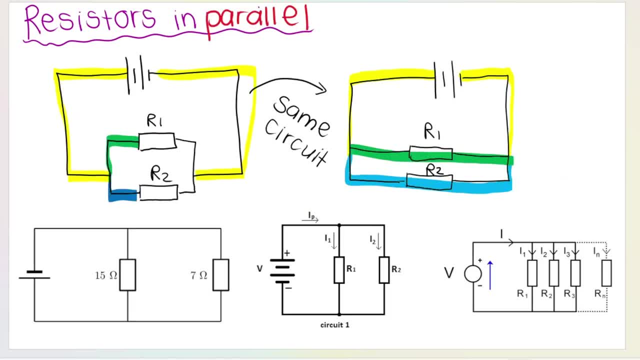 connected in series. A parallel connection is quite obvious to see This and this over here is representative of the same circuit. The reason I drew both of them is because in some exams, in some textbooks and some study guides you will see it being represented like this: 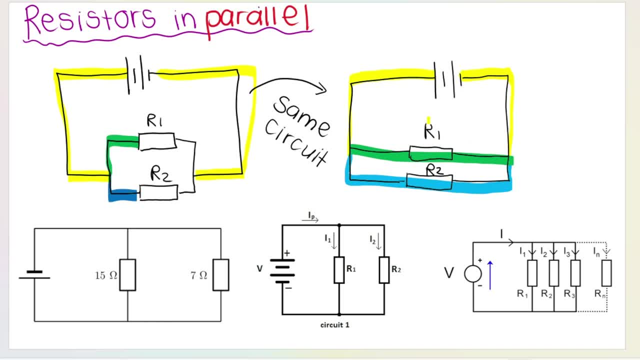 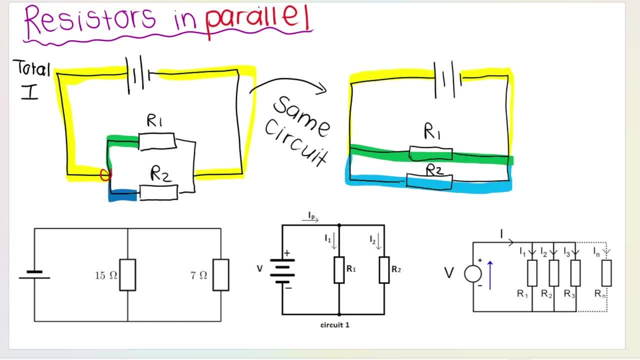 and then at this point over here, which I will indicate with a red dot, we can see that there's a split in the main line of the circuit. Some of the current goes through the top branch, so in other words through R1, and some of the current goes through the bottom branch, through R2.. Then 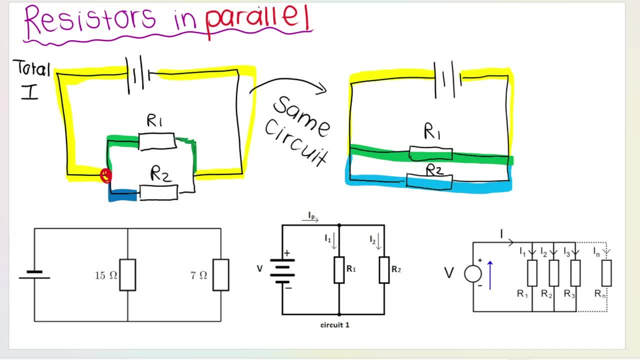 they join again. So this is a split in the main line of the circuit. This will still be R1 over here, On this side over here. this will still be R2 over there. and then, once again at the red dot, they join and it becomes total current again. 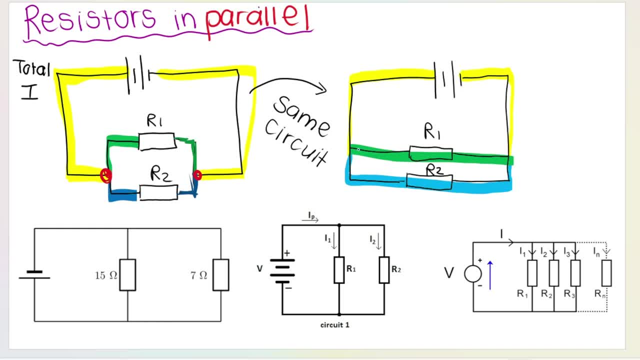 This is the same thing, except the branching is just drawn a bit differently, So it splits there and there R1, R2.. This is basically the same representation: Total current, total current, total current. Then there's a split. Some of the current goes through this branch, the 15 ohms. 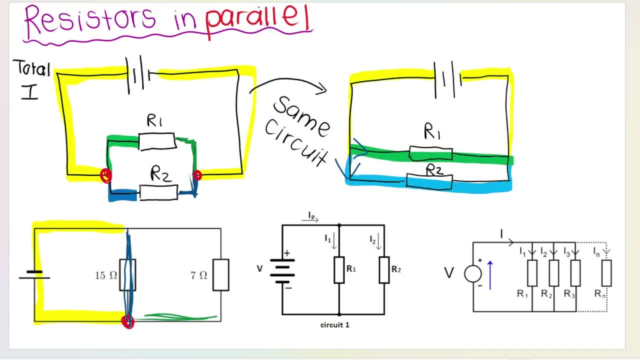 and the rest of the current goes through the 7 ohm branch like this, And then they join up again at this point over here. And these circuits over here represent the same thing. It's just that over here there are three resistors in parallel. Now how would you calculate resistance in parallel? 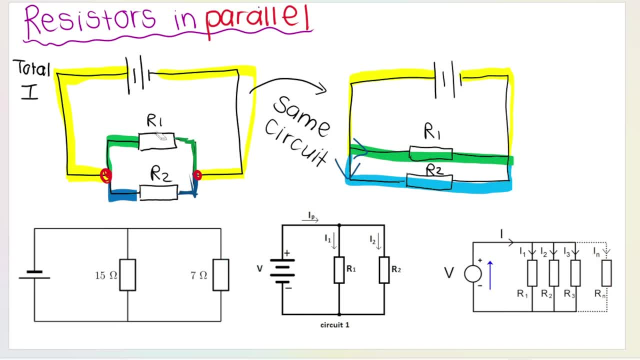 I mean, if I had to do the circuit over here at the bottom, because it actually has values, what I would do is I would say 1 over RP, because these are in parallel, 1 over R1 plus 1 over R2, R1. And I want you to think of R1 as being this branch. 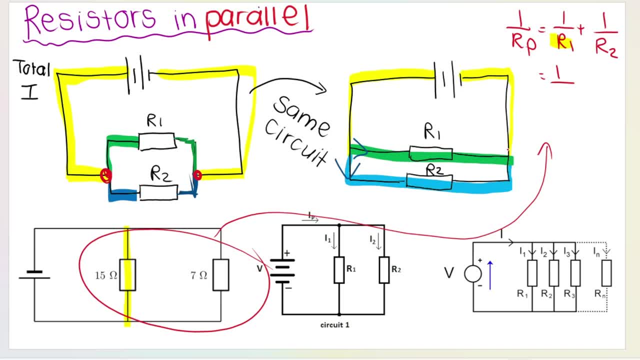 What is the resistance of this branch? This branch is 15 ohms, so it's 1 over 15 plus R2.. I want you to think of R2 as being this branch. Which resistors are in that branch? Just the 7 ohms. 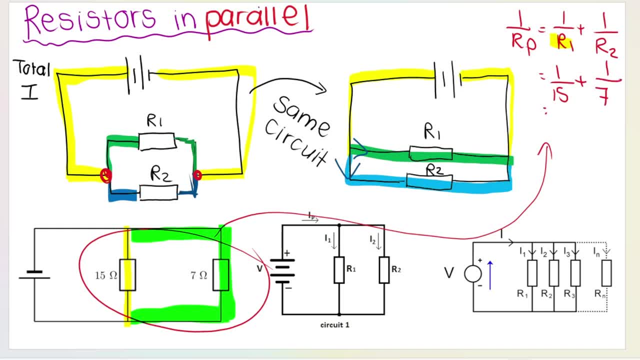 so it's 1 over 7.. Then what you do is you type it as is on your calculator like that: 1 over 15 plus 1 over 7. It's a bit of a terrible number, but you get 22 over 105.. But please- and I will do this again in a later question- 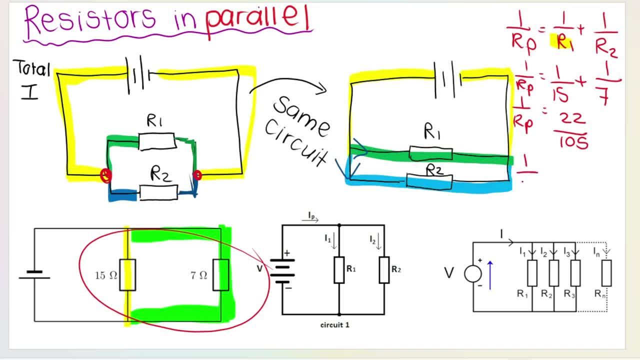 take note that. let me write it a bit nicer. this is 1 over RP, is 22 over 105.. I just typed 1 over 15 plus 1 over 7 on my calculator. I do not want 1 over RP, I'm looking for. 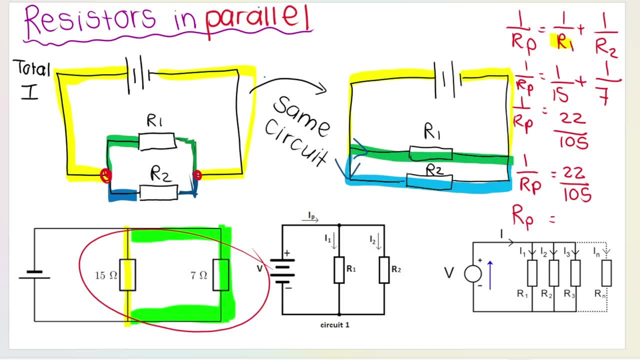 RP resistance in parallel. So what I need to do is I need to flip this fraction. So take the reciprocal or flip this fraction. Because I'm flipping this fraction, I need to do the same thing to the other fraction. So it's going to be 105 over 22.. And you can work that out on. 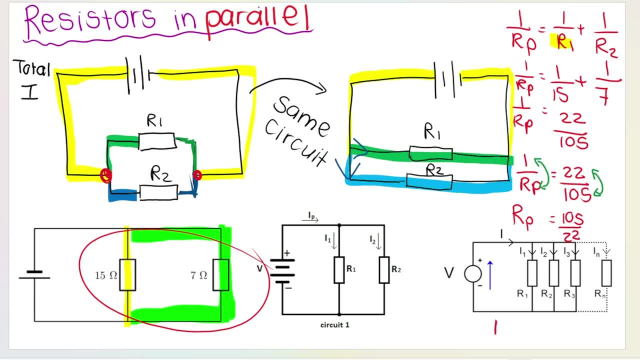 your calculator, 105 over 22. And I get RP as being 4 comma, 7, 7 ohms. Okay, so you flip this fraction. flip this fraction and then work out an answer. Remember, write it to at least two decimal places. and there's my unit. Now here are some other circuits. 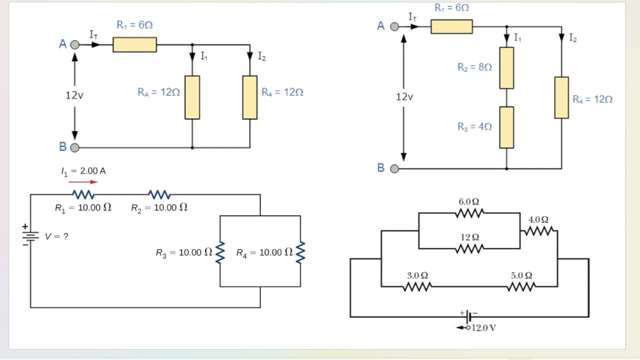 And I hope that you can recognize that this is a combination. These circuits are combination circuits. In other words, we have a resistor that is in series and we have resistors that are in parallel. I know that these circuits look a little bit different to what you're used to. 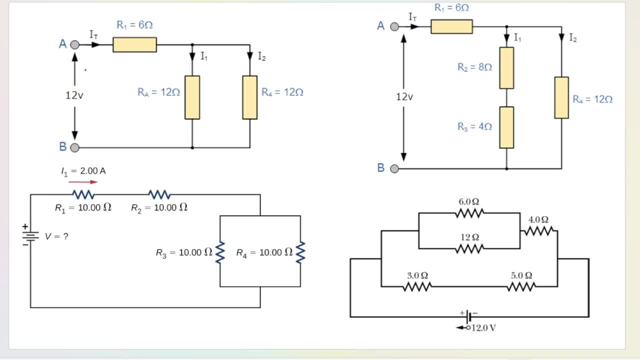 seeing, maybe in textbooks, study guides or in past papers. They come from the internet, but it's basically the same thing. Let's see, This is the battery. So you see, it says 12 volts. This is where your battery would be connected. So let's just draw a battery with two cells. 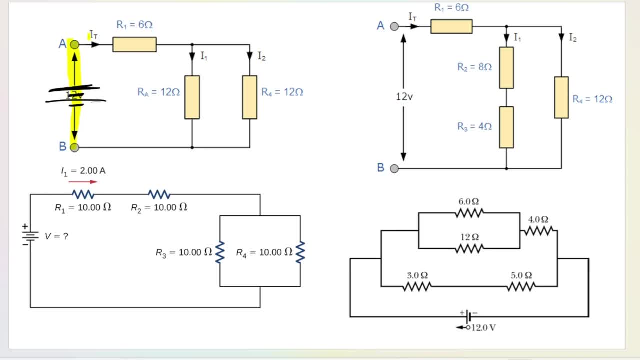 This is the main line of the circuit, So the total current will flow. You see, it says IT total current. The total current will flow through R1.. Okay, then I hope you can see that there's a split in the circuit there. I've got a branch. 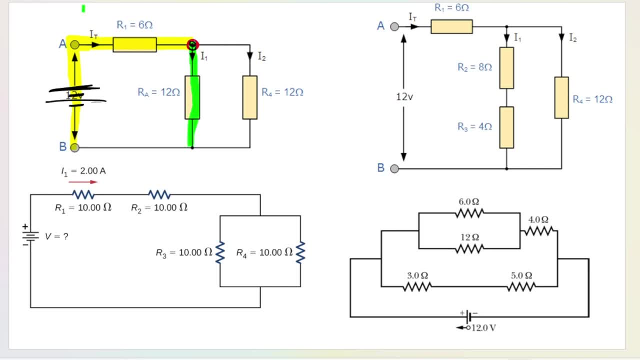 and there's still a branch going on here. Let's go back to the previous sequence. There are two toudensterns in the inside here. The two will be transferred to each other four side, but the total current will go through R1.. feeding through this part of the circuit. 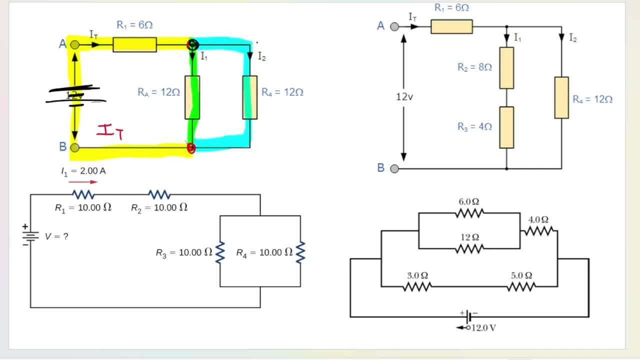 And then the total current will go through this branch. The rest of the current will go through this branch- are in parallel and this resistor is in series. so how would i work out the total resistance of this circuit? well, i want you to always start off with any parallel resistors. always start off with 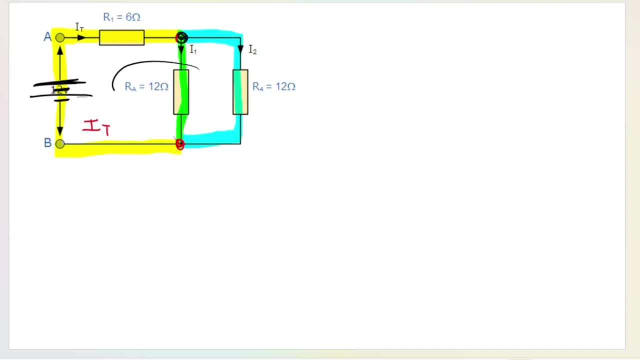 a parallel combination and, as we discussed, this resistor over here, the 12 ohm- and this resistor over here, the other 12 ohm, they are in parallel and the way that we know that is because some of the current goes through this branch, the green one, and some of the current goes through the blue. 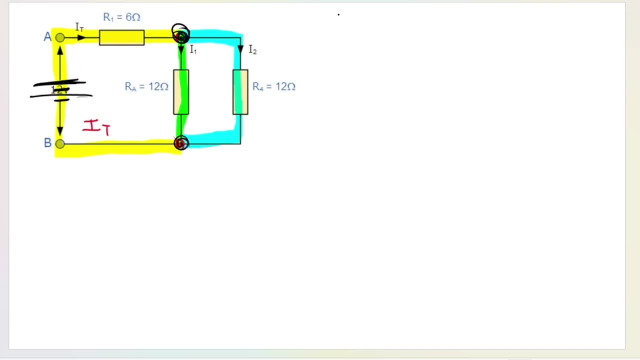 branch, so they are in parallel. there's a split in the circuit. so what we need to do in order to calculate resistance of the circuits, i'm going to write your resistance or total resistance. how we do that is, we start off with the parallel resistance, so we're going to go one over rp. 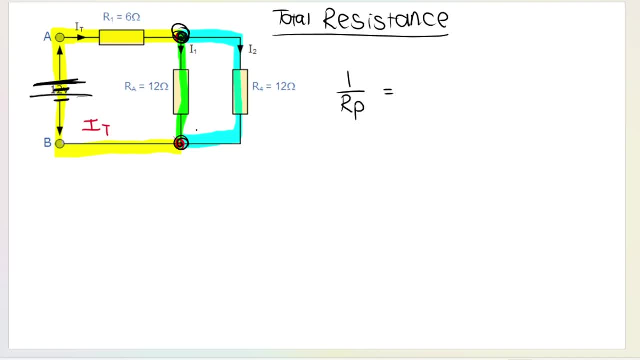 now, how many branches do i have? i have the green branch and the blue branch, so one over r1 plus one over r2. i want you to think of r1 as being the green branch and i want you to think of r2 as being the blue branch. that's my formula. you get a mark for writing your blank formula. 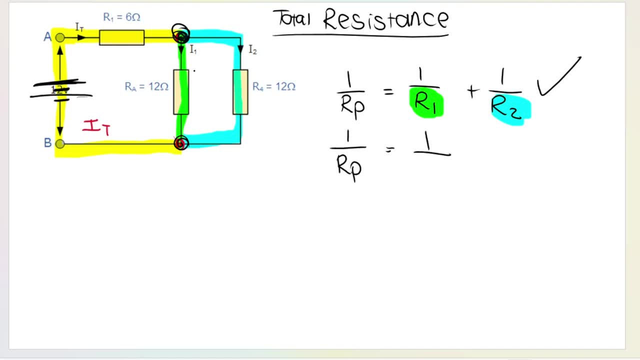 then what is in the green branch? what resistance is in the green branch? this one, 12 ohms, so it's 1 over 12, plus what resistance is in the blue branch. look at the blue branch. we've just got this one, 12 ohms, so 1 over 12.. basically, you can do that on your calculator, but this is a very easy. 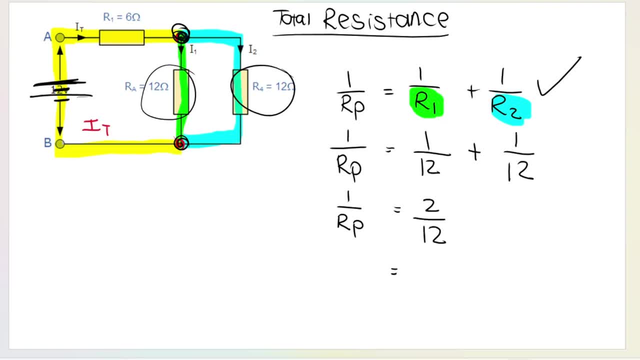 one. this is 2 over 12. and remember what i showed you. we don't want rp, we 1 over rp. we want rp, so we must flip that fraction so rp comes to the top. it's basically rp over 1 if we flip it. but rp 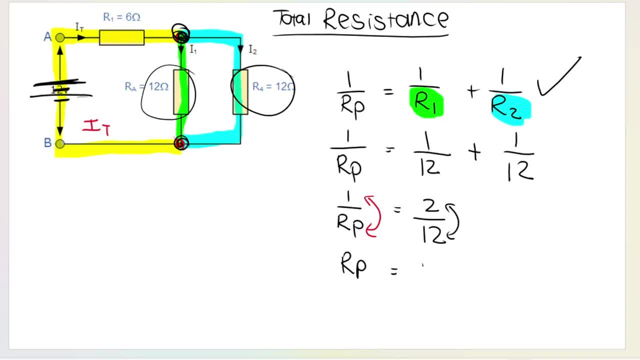 and then we flip this fraction as well, so it's going to be 12 over 2.. what's 12 over 2? it is 6 ohms. now, what you need to understand about this is what this means. is that sure? when the red Chinese character comes to the bottom, we go to the bottom of the blue order. 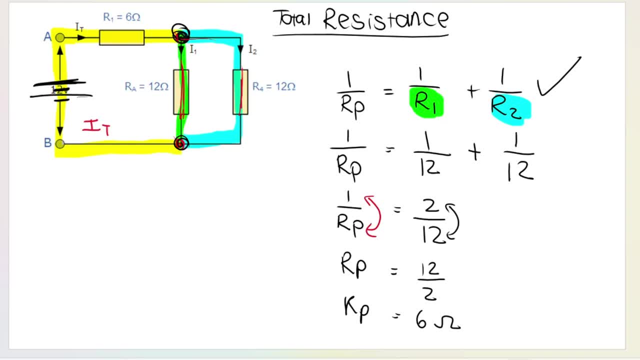 when the current splits. some of it goes through this 12 ohm. some of it goes through this 12 ohm Overall, this part of the circuit has a resistance of 6 ohms, So it's kind of like removing the. 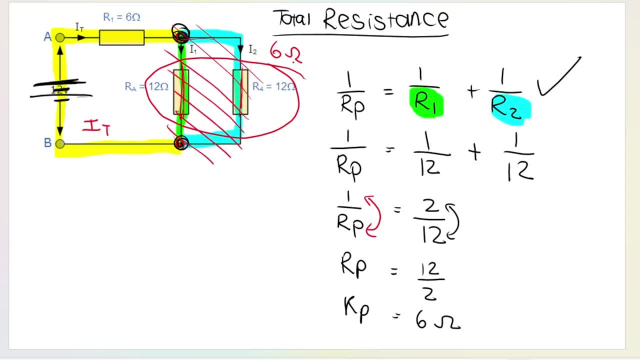 parallel section and replacing it with something that has 6 ohms will basically be the same as the situation that I have at the moment, where I have two 12 ohms in parallel. I hope that makes sense. So overall, this part of the circuit is 6 ohms, But remember I also have this resistor over here. 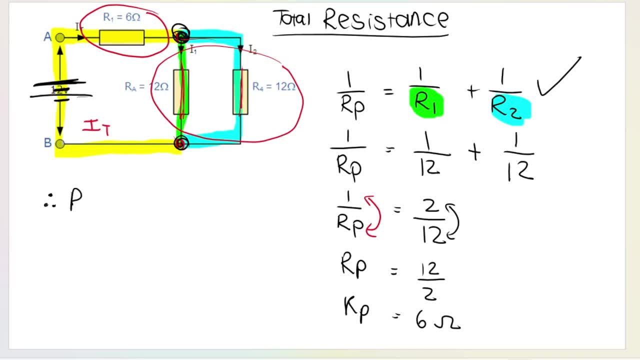 in series, this 6 ohms. So, therefore, my total resistance is this resistor, this 6 ohms. So the one I'm going to call it the yellow one, the one that I've highlighted in yellow, plus this 6 ohms, 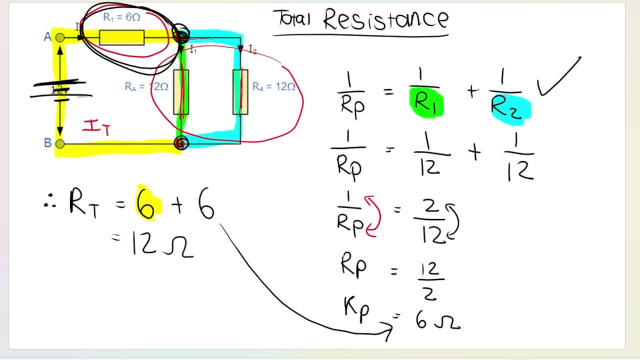 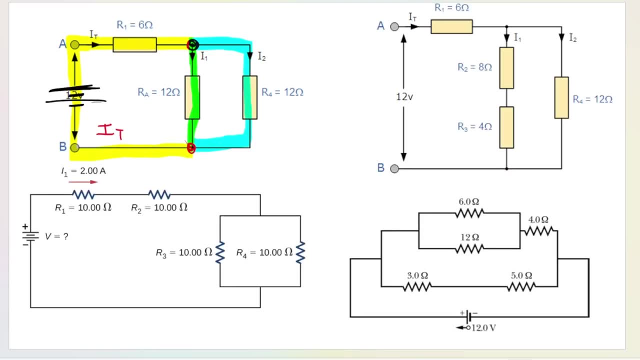 the one that I got over there. So my total resistance is 12 ohms. So you first work out the parallel, get an answer and then add any resistance That are still in series. Let's take a look at one more circuit, And this one can be quite 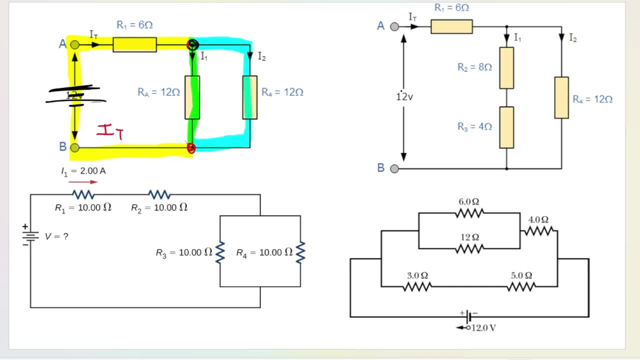 confusing. And it's this one here on the right. So if I have, this is my battery. Okay, there's my battery. once more, The total current will flow through the battery. The total current will flow through this 6 ohm over here And the total current will flow through here. But then I have a split. 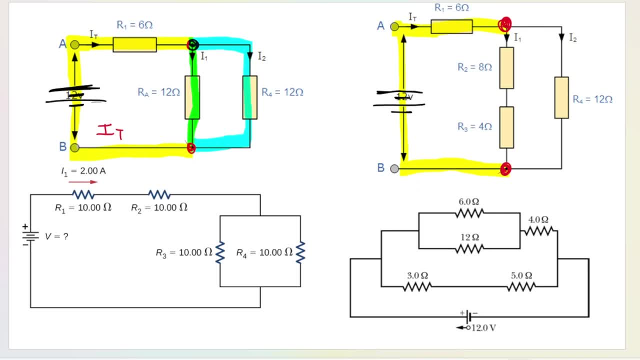 in my circuits There's the split and there's the split depending on which way you look. Some of the current will go through this branch over here. The rest of the current will go through this branch over here. So how do I work out the total resistance of this circuit? 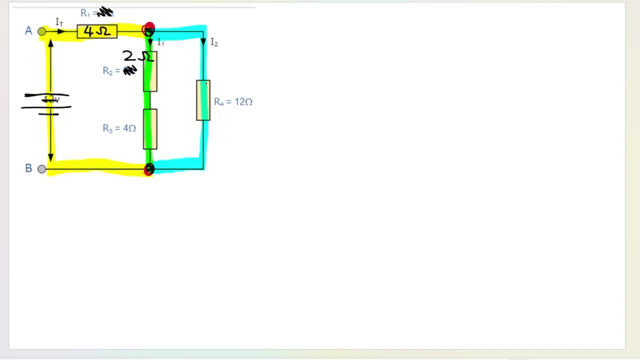 I change the values of these resistances just to keep it a little bit interesting, a little bit different. Let's make this one 10 ohms. I just don't want the same answer as the previous one. Let's make this one 4 ohms. So what we do first is we work out the parallel. 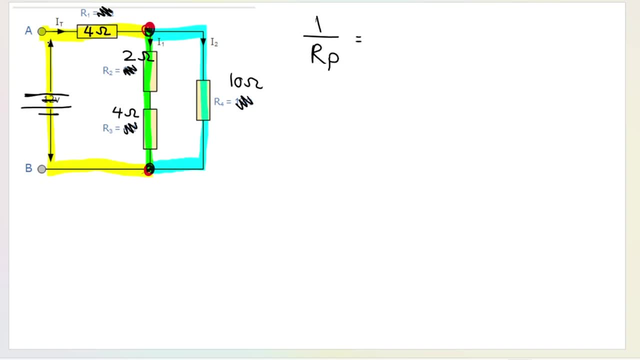 resistance. So what we do first is we work out the parallel resistance. So what we do first is we. and now I want you to remember what I told you in the previous example. I want you to think of 1 over R1,, 1 over R2.. I want you to think of each of these as a branch. Okay, I want you to think. 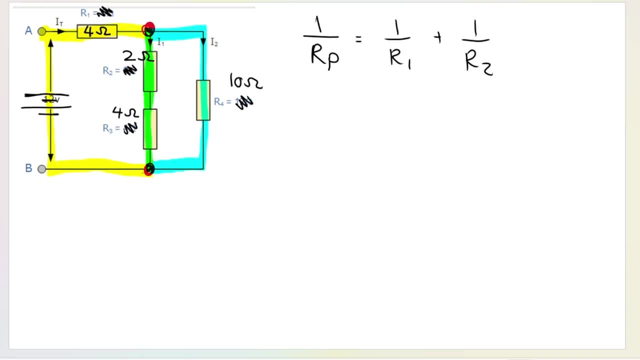 of each of them as a branch. So the green branch is going to be R1.. And I know that that's confusing because you're like, wait, ma'am, isn't R1 a resistor, So shouldn't there be two of them? 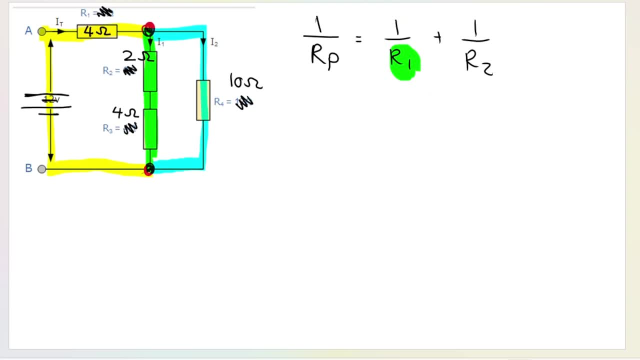 I want you to think of these things as branches. This is where a lot of my students they're wrong If they, when they don't think of it like this, think of the blue branch, this one, as R2.. Okay, So the wrong formula. wrong formula would be saying 1 over RP. 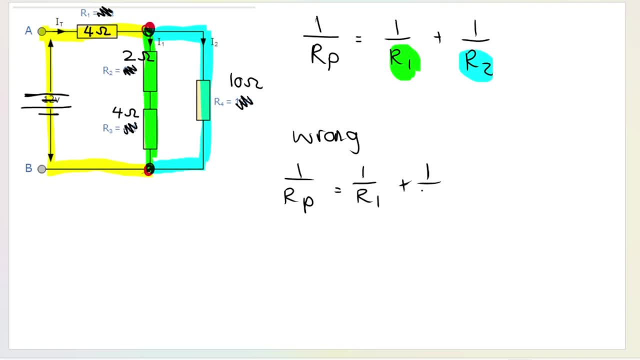 is 1 over R1, 1 over R2 plus 1 over R3.. And I know some of my students think that because there's 1,, 2, 3 resistors here. However, you will only use a formula like this if there are three. 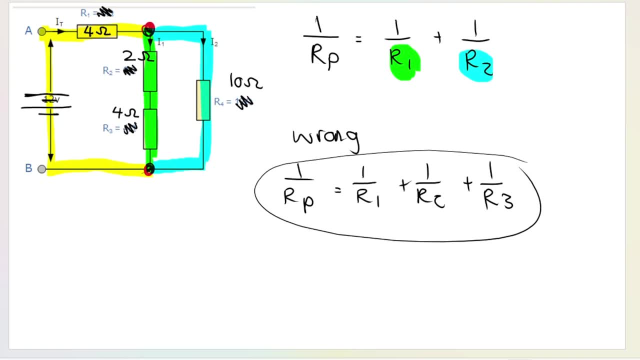 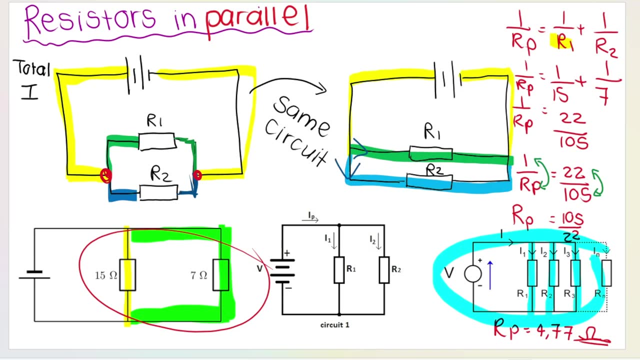 branches. So you'll only use 1 over R1,, 1 over R2 and 1 over R3, or a circuit that looks like this one, where there's 1,, 2, 3 branches, If we only have two branches, like we do in this example. 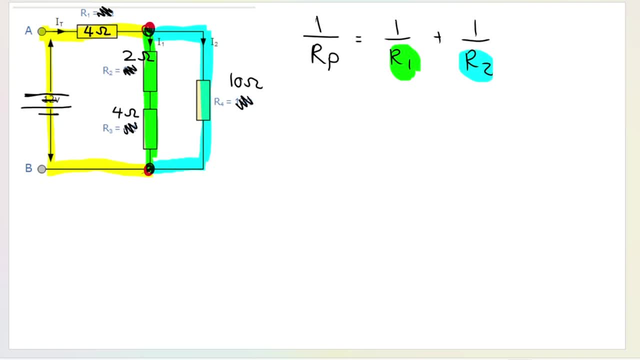 the green branch and the blue branch. we only have 1 over R1 and 1 over R2.. So R1 is both of these resistors together, 4 and 2 together. Why am I adding them like this? Because the 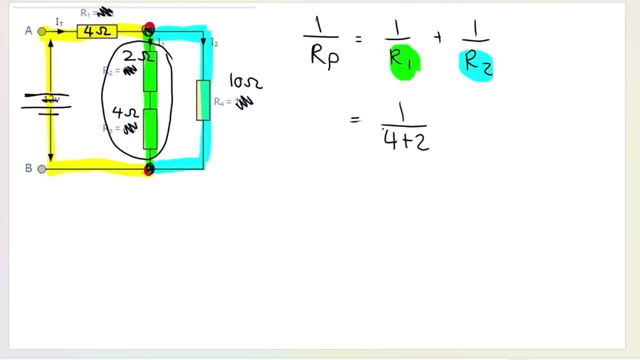 4 and the 2 are sitting next to each other. They're in series, So it's 1 over 4 plus 2.. Basically it's 1 over 6 because this branch has a resistance of 6 plus the blue branch. 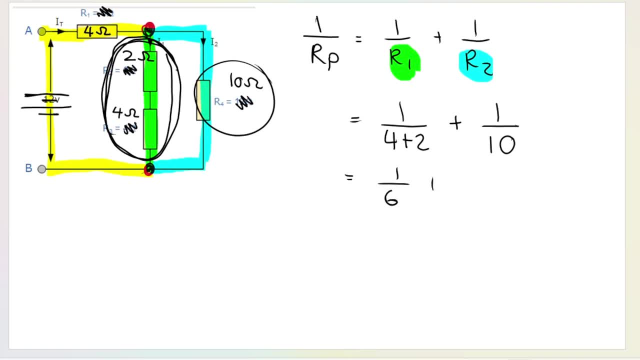 1 over 10.. So it's 1 over 6 plus 1 over 10.. I want you to use your calculator to do that. You don't need to do it manually. And we get 4 over 15, but remember we must flip both fractions. 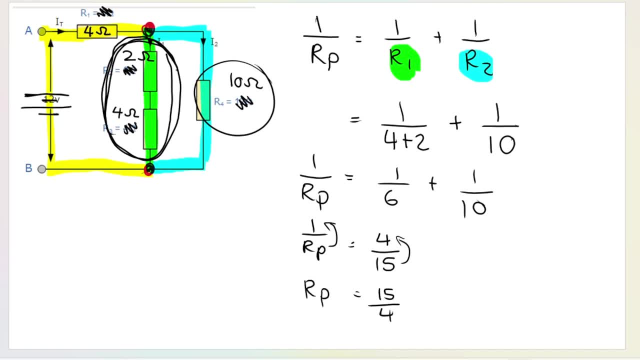 So RP is 15 over 4. Ohms- If you want to write that as a decimal, you can. So 15 over 4 is 3,75 ohms. Now, what we just calculated is the resistance of the parallel connection. So this thing basically has a. 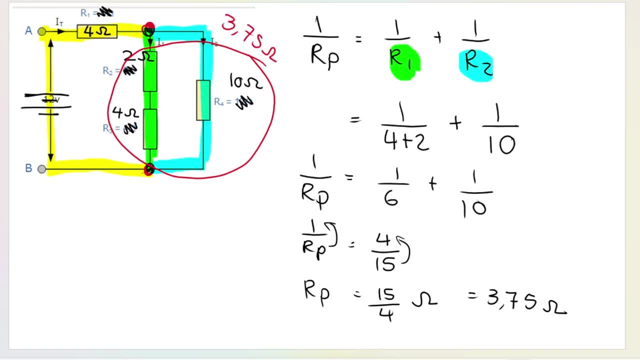 resistance of 3,75 ohms. But remember we are looking for the total resistance of the circuits, So we must still add this resistor in series. So the total resistance is 3,75, which is 3,75 ohms. So we're going to add this resistor in series, So the total resistance is 3,75,. 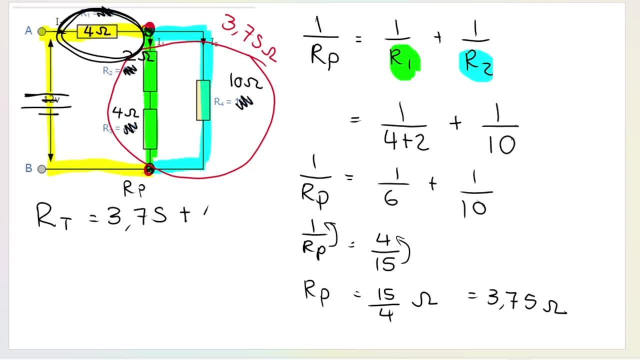 resistance in parallel plus 4 ohms, which is basically my resistance in series, And we get 7,75 ohms. So once more you work out the parallel, then you add what you have in series. So if there were two in series, say there was another 4 ohms, then you would say 3,75 plus 4. 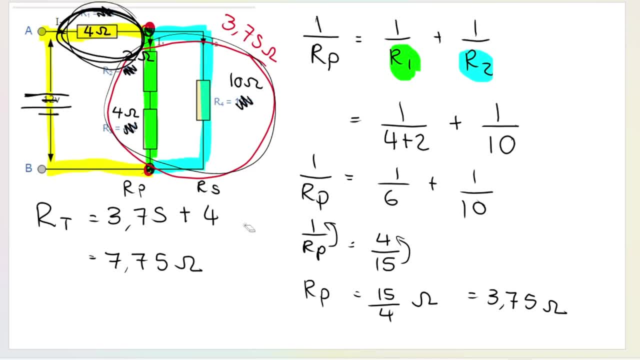 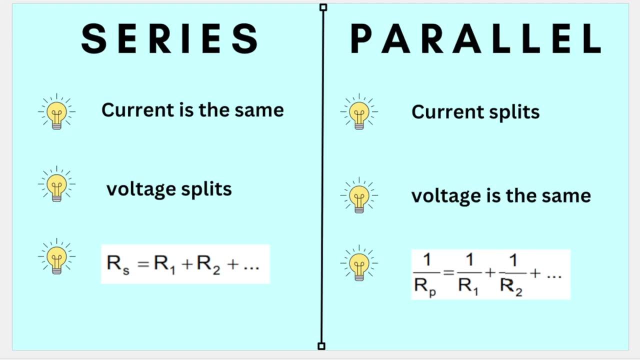 plus 4.. But we only have one in series. We don't have that one, So that's why it's just plus 4.. I hope that makes sense. Let's move on. So understanding series versus parallel circuits and what happens to current and what happens to. 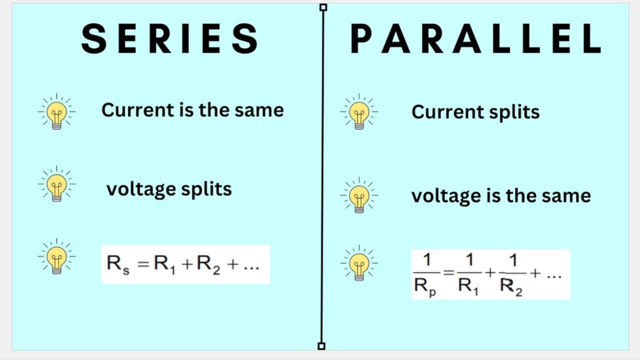 voltage within these circuits is very, very important. So on the screen you can see a summary of that. And the two most important things to remember is that in a series circuit, current is the same everywhere, everywhere, throughout the circuit, but voltage splits. 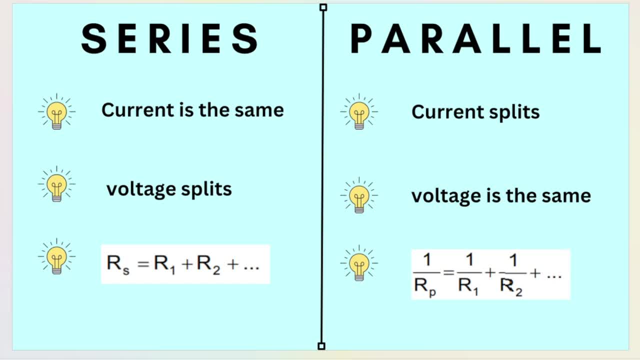 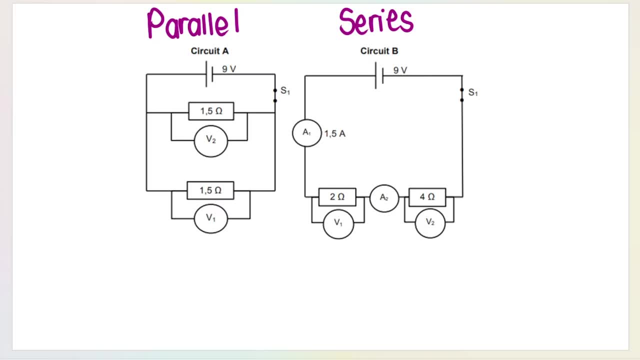 In parallel. the opposite is true. So the current splits and voltage is the same for resistors connected in parallel. So if we compare these two circuits over here, let's look at the series circuit first. What it means is: do you see that the ammeter over here measures 1.5 amperes? 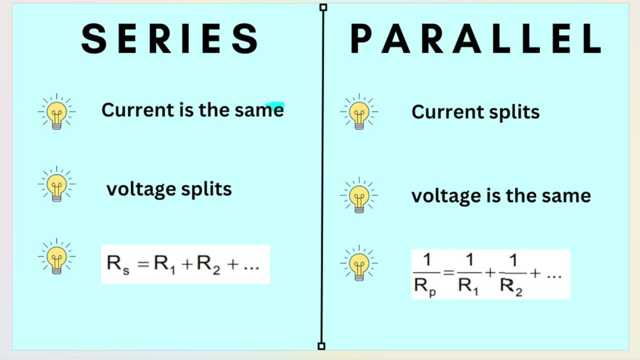 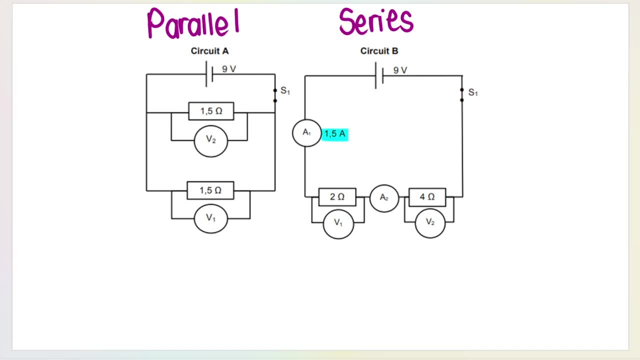 Now remember we said in series: current is the same everywhere in the circuit. What that means is the total current is 1.5 amperes. So 1.5 amperes will flow through the battery, 1.5 amperes will flow through the ammeter, 1.5 amperes will flow through. 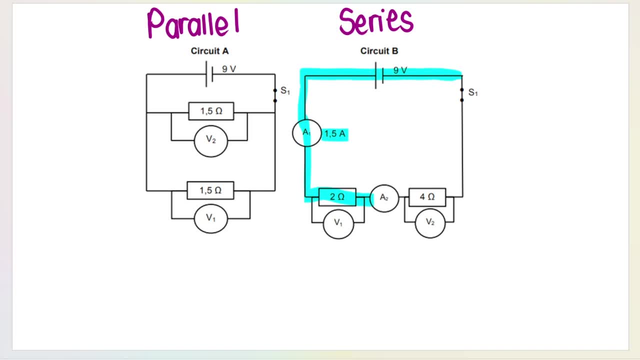 the 2 ohm resistor. The reading on A2, the reading on this ammeter is 1.5 amperes. 1.5 amperes flows through the 4 ohm resistor. 1.5 amperes flows through here and back to the battery. 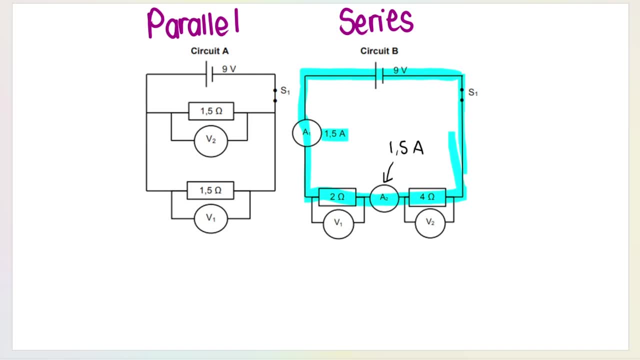 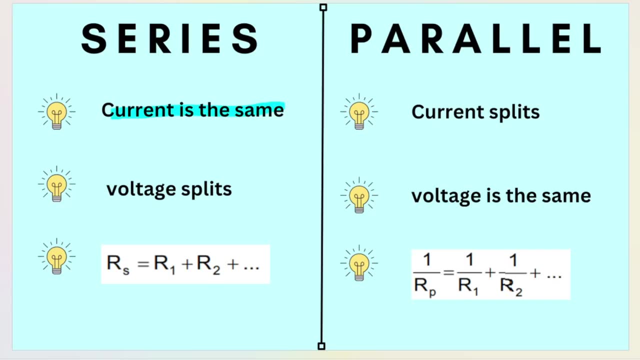 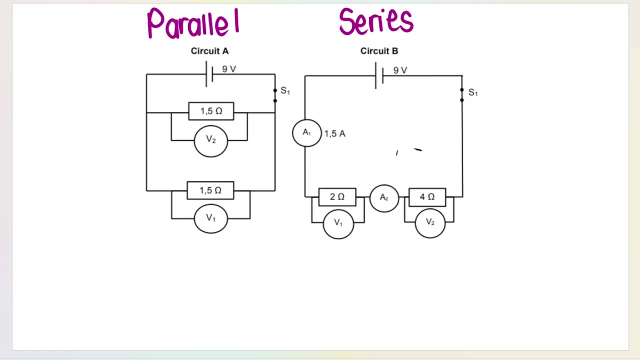 There are no splits in the circuit, There are no resistors connected in parallel, So current is the same throughout. So that is what it means by current is the same, However, voltage split. So what that means- and I really, really want you to understand this carefully- What that means is: 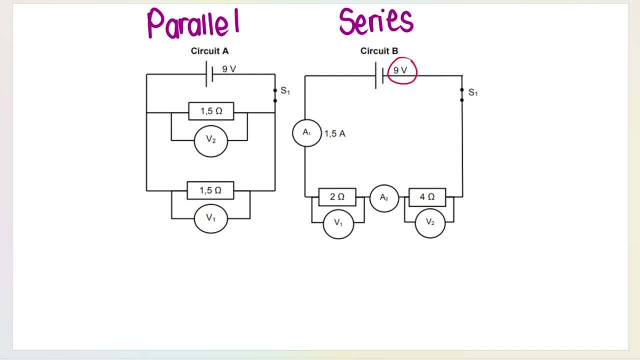 the voltage across the battery. you can see here it says 9 volts. So what that means is if I had to connect a voltmeter across the battery like this- remember- voltmeter reads potential differential voltage. If I had to connect a voltmeter across that battery, it would read 9 volts. 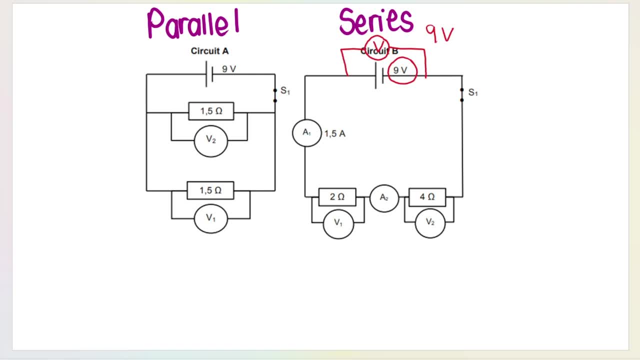 Now that 9 volts is the total voltage, total potential difference or external or terminal potential difference- Okay, terminal potential difference- and that 9 volts is split amongst the different resistors or components in series. So some of the 9 volts will go here and the 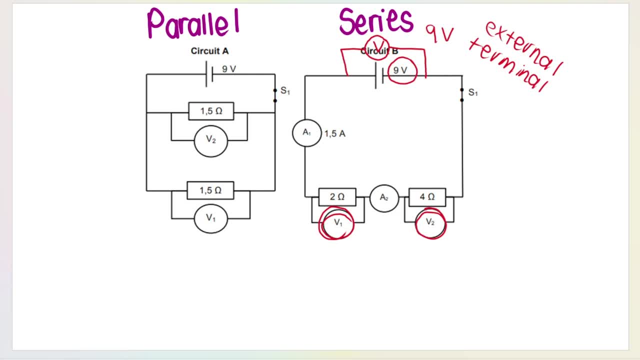 rest will go. here We can actually work out much voltage will go to this resistor. i hope you remember the formula. v is equal to i times r, remember i is current, the total current, well, the, the total current flows through this resistor, so 1.5 amperes. 1.5 amperes flows through that resistor and the resistance is 2 ohms, so that 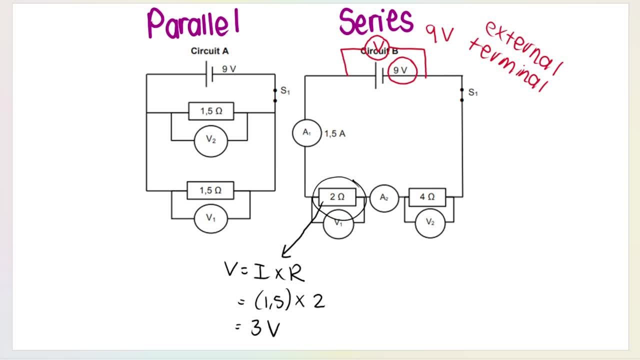 means that the voltage v1 is 3 volts. so what that means is that when v1 has a reading, v1 will read 3 volts. if i had to do a similar calculation, but for this resistor over here it will be: v equals i times r. current once more is 1.5. remember the total current, 1.5 flow through. 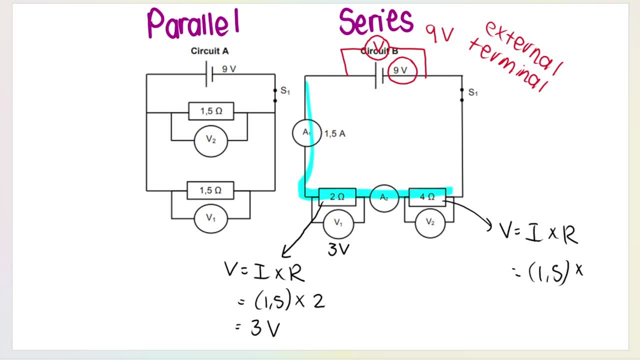 both of these resistors times. the resistance over here is 4, and 1.5 times 4 is 6.5 amperes, 6 volts. so this volt meter over here will read 6 volts and i hope you can already see what's. 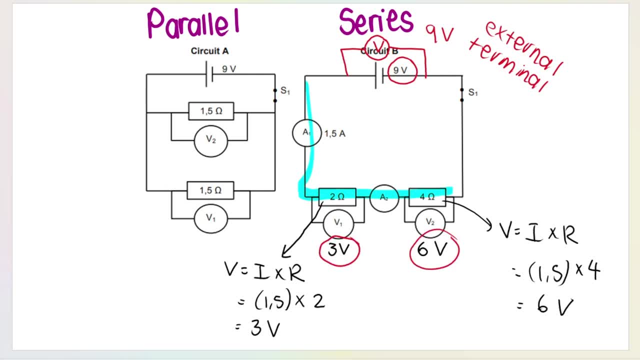 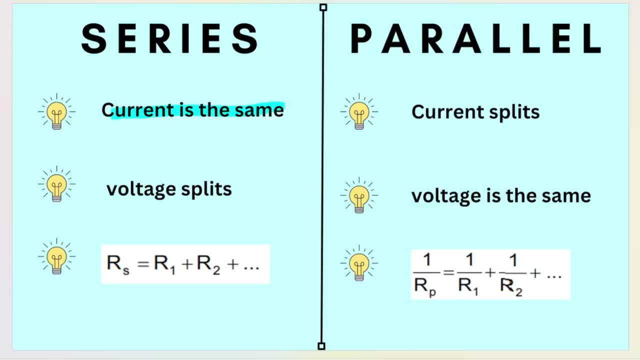 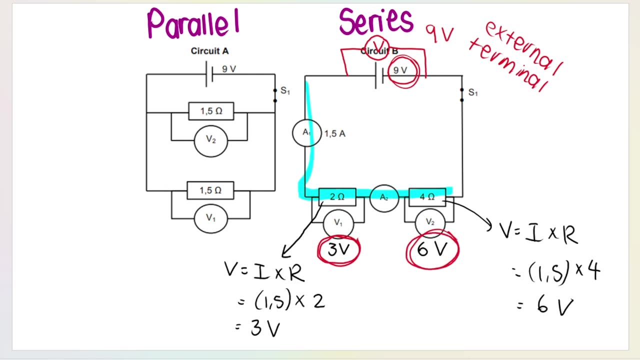 happening. if i take 3 volts plus 6 volts, it gives me 9 volts and that just shows me that voltage in series is split, just what it says there. so of the 9 volts across the battery, 3 volts goes here, 6 volts goes here. 3 plus 6 is 9 volts. let's look at the parallel circuit. parallel circuit is the. 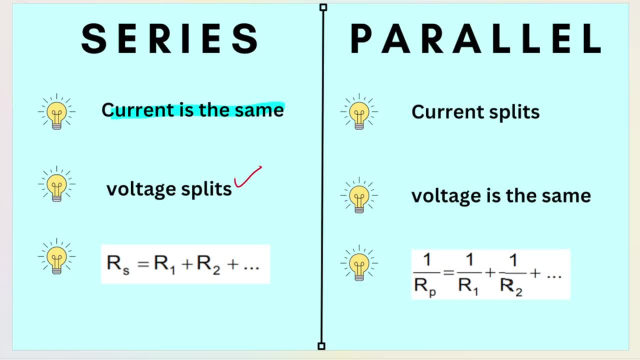 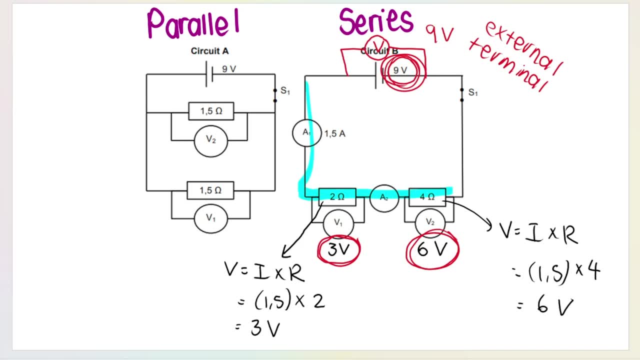 opposite current split in the parallel circuit. so what that means is, if we look at the parallel circuit, the total current will flow here because these parts are in series. the split has not happened yet, so this would be total current, total current as soon as you get to a split, as you can see here. 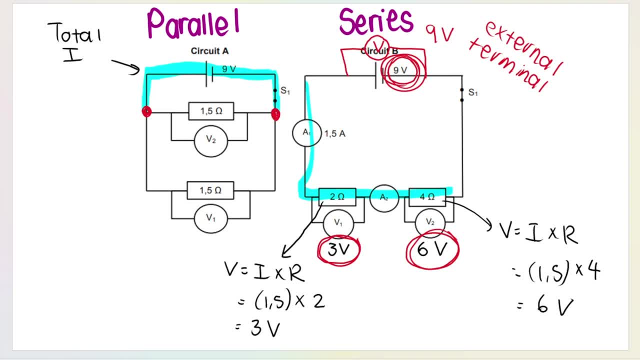 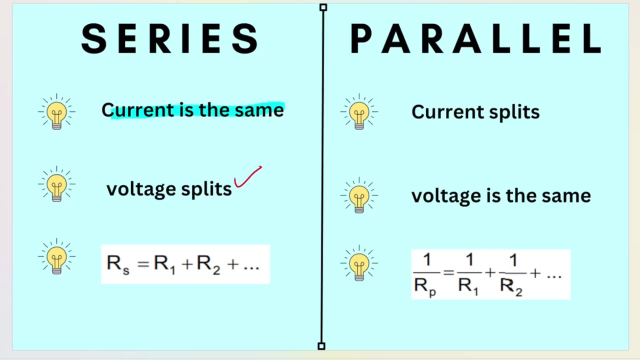 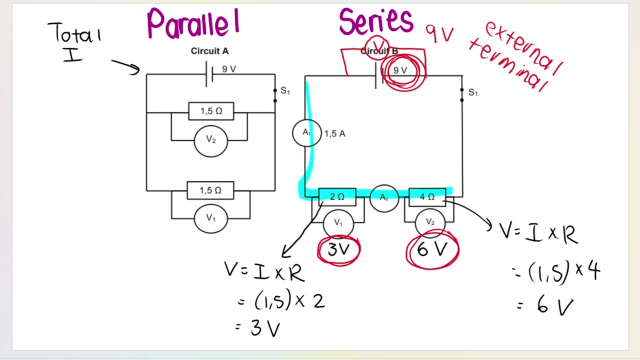 the circuit line splits as soon as you get here. if you go this way, that's the circuit line split over here, so it's split or wave over here. when i go this way, i can see that some of the current goes through here, as i've mentioned. 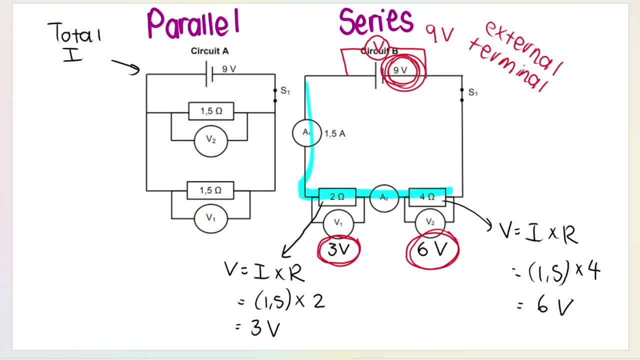 previously in this video and some of the current goes through here. so current voltage across this 1.5 ohms is the same as the voltage across this 1.5 ohms and in this case those voltages will be the same as the voltage across the battery because they're all in parallel. 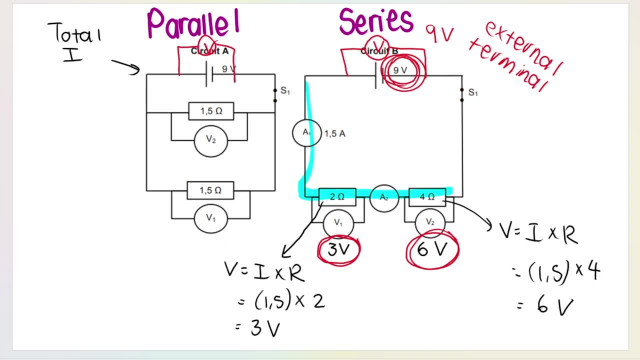 so the battery. if i had to attach a voltmeter across the battery, it would read nine volts, because it says nine volts over there. that means that v2 would read nine volts. that means that v1 would read nine volts. that is because in parallel voltage is the same across parallel resistors. 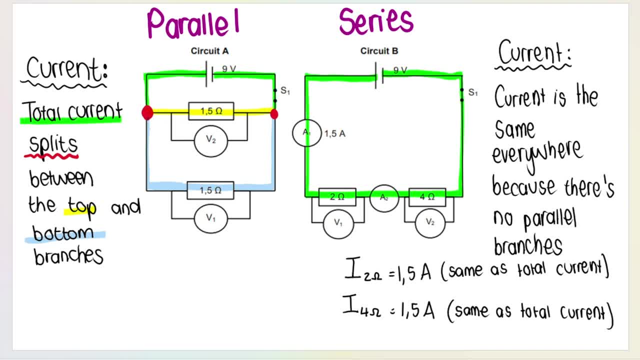 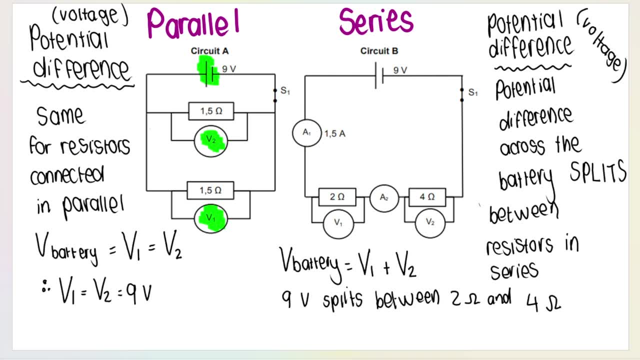 so here's basically a summary of what i just mentioned. okay, for current, and here's a summary of what i mentioned for voltage. so how we could represent this mathematically for parallel is the voltage across the battery. nine volts is equal to v1, which is equal to v2. they're all equal to. 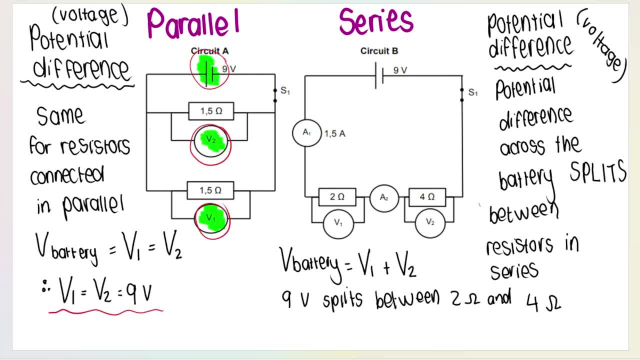 nine. for the series circuit, the voltage across the battery is equal to v1, which is equal to v2. they're all equal to nine. for the series circuit, the voltage across the battery is equal to v1, which is equal to v2. they're all equal to nine. for the series circuit, 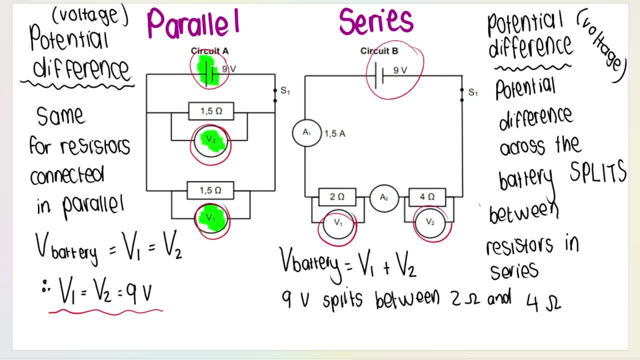 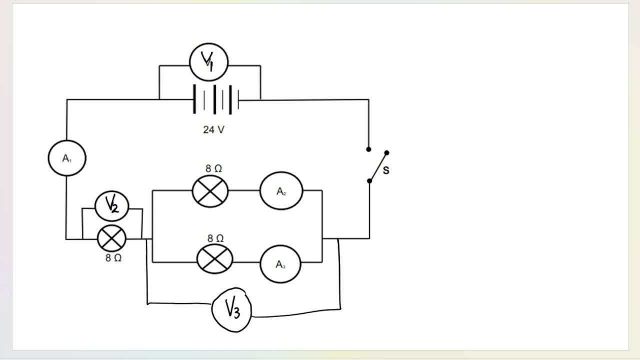 the battery, which is nine volts, is equal to this voltage plus that voltage. but what about when i have a circuit that looks mixed like that? and when i say mixed what i mean is, i have parallel resistors over here, so the eight ohms and the eight ohms are in parallel, but we also have 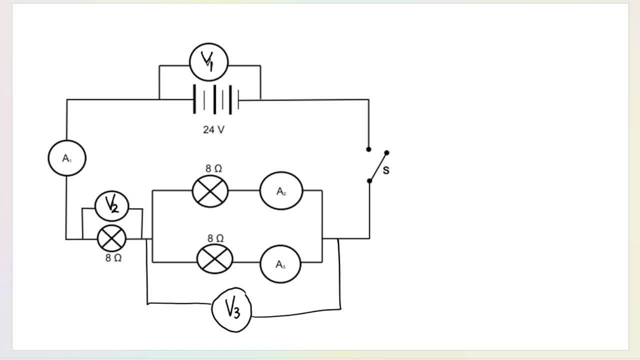 another eight ohms over here. that's in series. so how it works is as follows: the total current will flow through this part of the circuit, so a1 will read total current. the total current will flow through the resistor in series. then when i see a split in the circuit over here, we know. 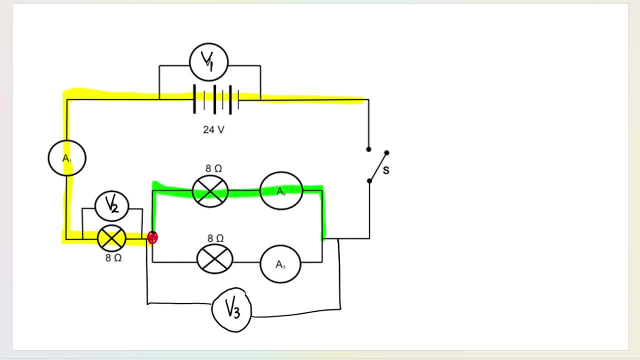 that the current will split. some of the current will go through the top branch and the rest of the current will go through the bottom branch and then they join again over here and then the total current will flow through this part. of course, this will only happen when the switch is closed. 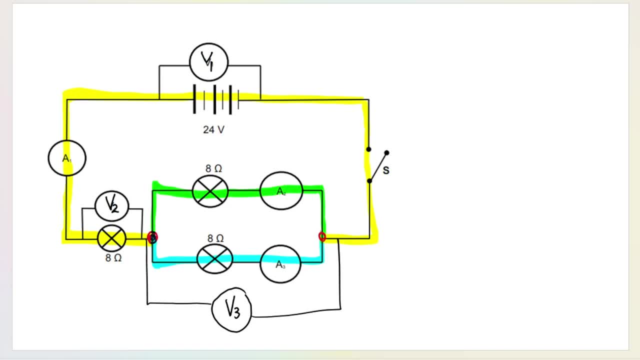 so just bear that in mind. so that is what happens with current, and i hope that you can be aware of the fact that. so a1 will read total current. it'll read total current. a2 will read a split current. a3 will read a split current. but what this means is if i had to take this current, the current reading on a2. 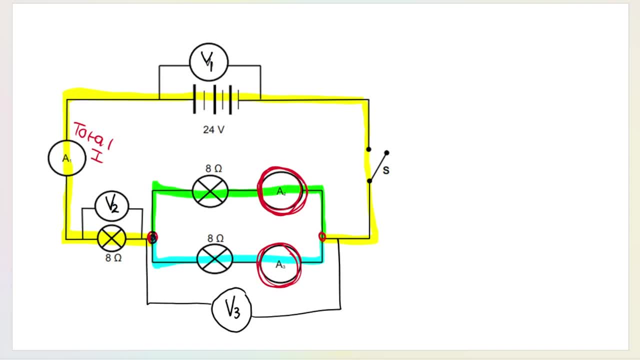 and the current reading on a3 and i had to add them together. it would give me the total current. so basically, the reading on a1 is equal to a2 plus a3, so the current, the total current, is equal to the current in the top branch, so the current in the green branch, let's say, plus the current in the blue. 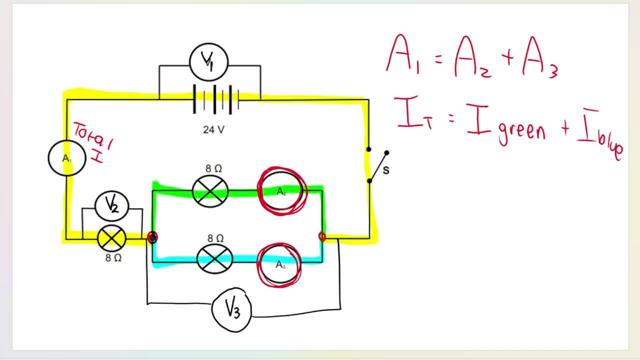 branch. i hope that makes sense. so current splits as soon as we have resistors that are connected in parallel for the voltage. what happens is quite interesting, and what happens is the following: you can see that we have v1 over here, so v1 measures the total voltage or total potential. 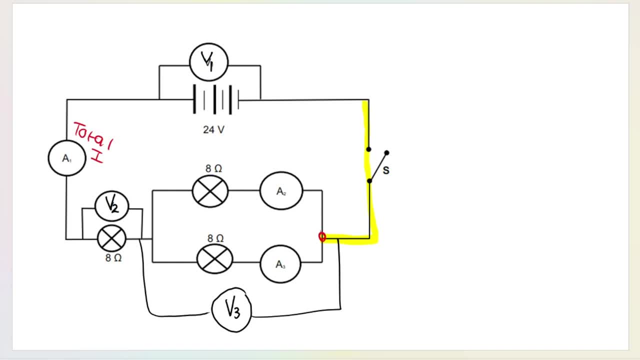 difference, or terminal potential difference, like we like to call it, and then we have the current. so v1 basically reads the total voltage or potential difference. now remember voltage splits in series. now, what that means is that you see, we have this resistor over here in series, and then we 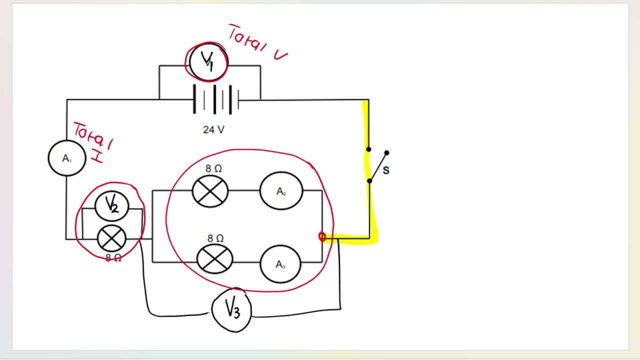 have what we call the parallel connection. now i need you to understand that. let's pretend i'm just making up numbers over here. well, i see here v1 is 24 volts. we can probably work out the the actual amounts here. i'm not bothered by actual amounts, but i'm going to work out the actual amounts here. 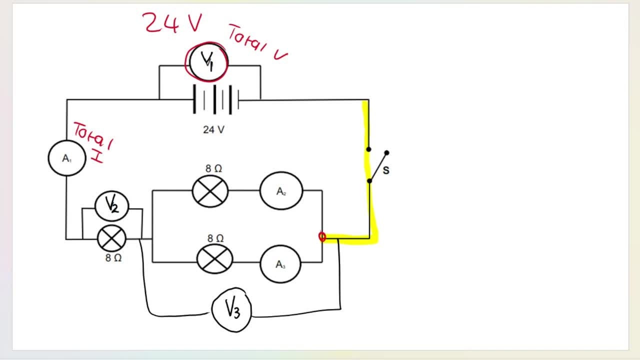 i'm just going to use make make believe amounts just to illustrate this concept. so say v1 reads 24 volts, then if v2 has to get- let's pretend it is 10 volts- that means that the parallel combination will get the rest, so it will get 14 volts. i hope that makes sense because the total voltage v1. 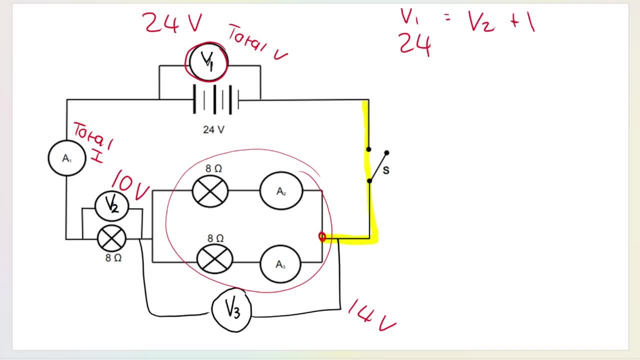 is split between v2 and v3, so v2 is 10 volts, v3 is 14. 14 plus 10 gets you 24, remember? i just made up these amounts and now you might be saying: okay, um, i'm not really sure if i understand, ma'am, because 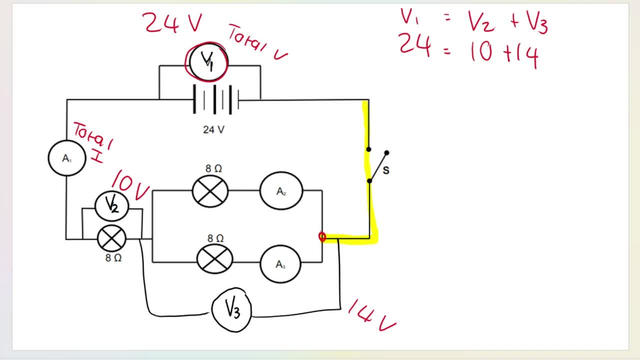 these are in parallel. so what does that mean? doesn't that mean that they get the same voltage? so wouldn't it be 7 and 7? no, remember. how i want you to think of it is as follows. think of it as this: 8 ohm is connected in series. 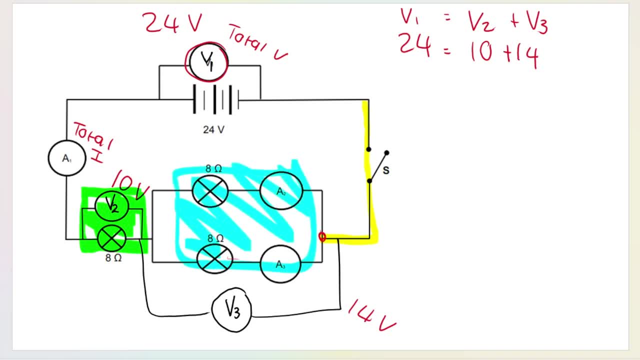 almost with this parallel connection. okay, so the green part of the circuit is connected in series with the blue part of the circuit and we know that voltage splits in series. so this part of the circuit gets 10 volts. this part of the circuit, which is the parallel part, gets 14 volts. and what? 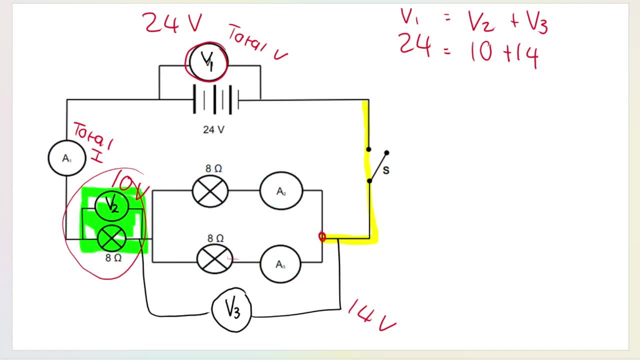 do we know about voltage in parallel? if we go back to our summary that i showed you over here, voltage is the same in parallel. so all that means is that if the voltage across the parallel connection is 14 volts, it means that the voltage across this 8 ohm resistor is 14 volts and the voltage across this 8 ohm resistor is 14 volts. 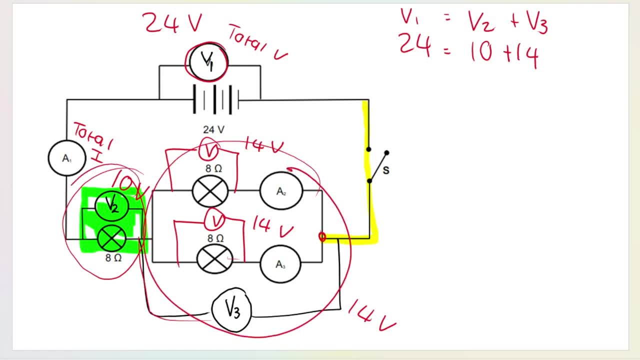 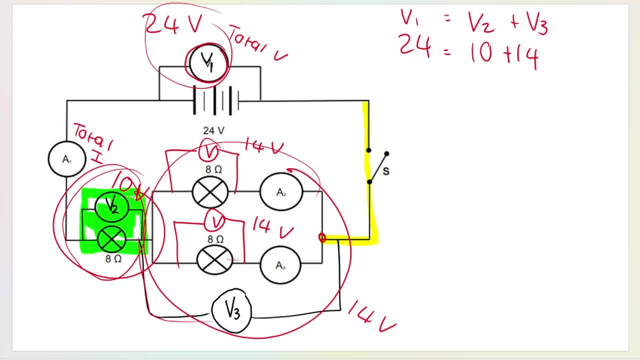 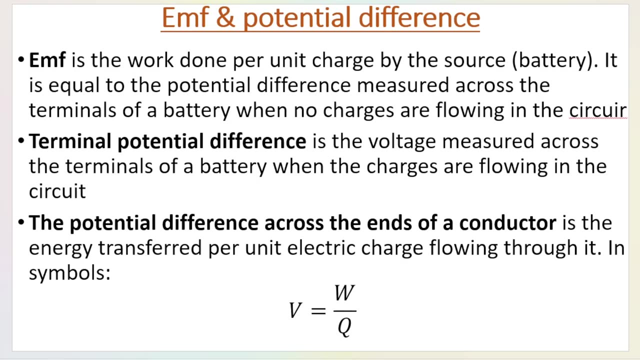 okay, so 14 over all over here plus 10 gives me the 24, and understanding that is actually really, really important for answering circuit calculations. now let's jump into using some of the formulae. what i've basically done is i've copied and pasted important definitions that you may see. 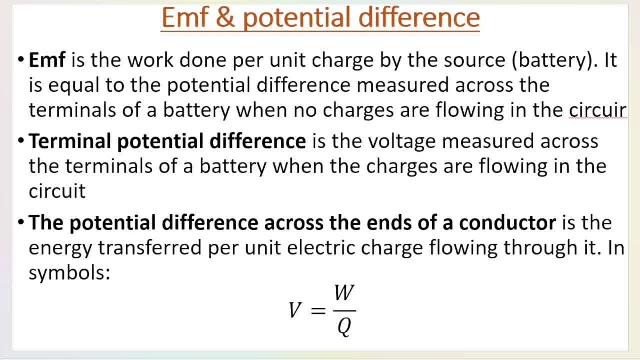 in your textbook, in your exam guidelines and such. so we've got emf, which is going to come into play in grade 11 and 12 more, but i want us to focus on all of these as being definitions for voltage potential difference. okay, and i want you to see the following. i showed you this formula. 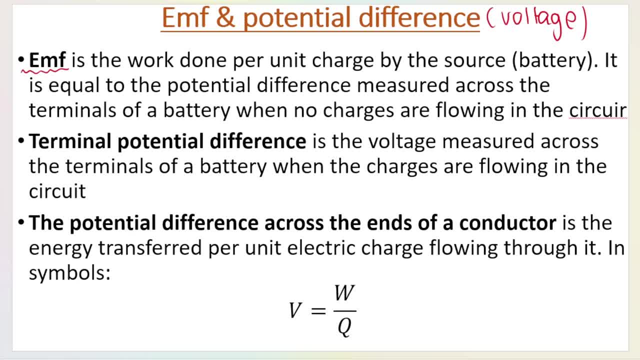 earlier in the video. but look at how it connects to our definition. the potential difference across the ends of a conductor is the energy transferred, and remember we said energy transferred is the same thing as work done. okay, so energy and work is the same thing, so it's the energy transferred. 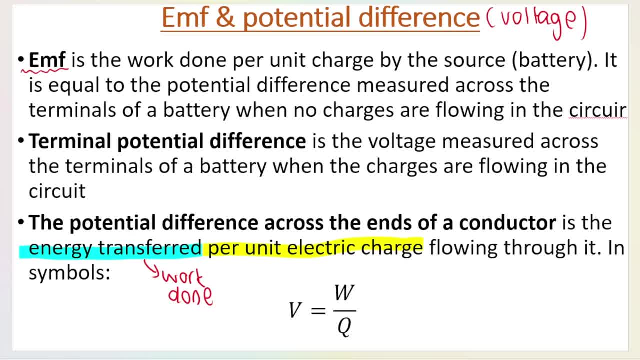 per unit electric charge flowing through it. now, if you take a look at that in words- so the definition- and you look at my formula, they match. so potential difference is v. there's v. potential difference is equal to energy transferred. remember w is the same thing as energy transferred. it's work done. 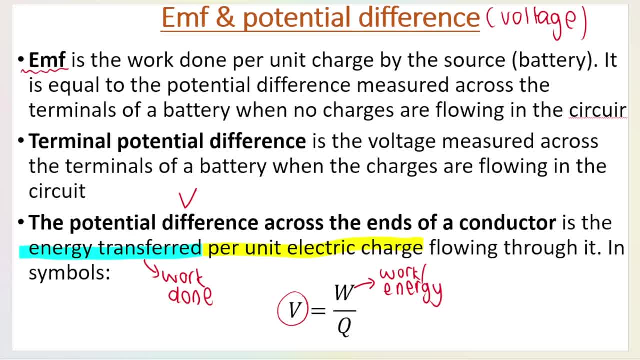 or energy transferred. so it's equal to the energy transferred per. when you see per, i want you to think of divide per unit electric charge and q, we know, is charge. so again, look at the formula, look at the words. they match. so potential difference is equal to the energy transferred or the work done. 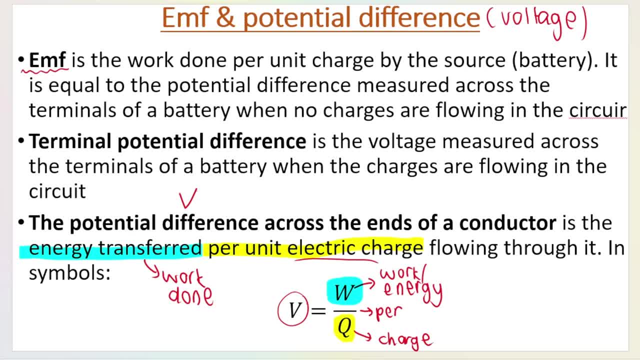 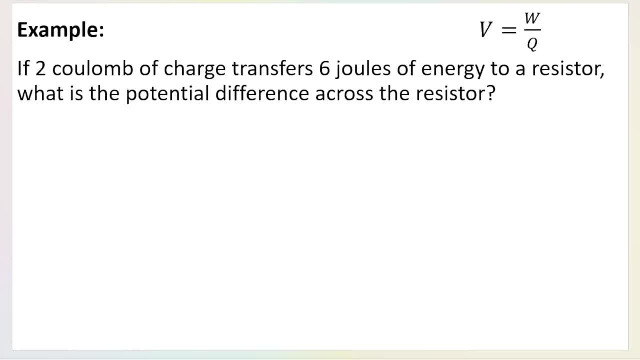 per, which means divide unit electric charge, and it matches with our formula. so this is a very basic example of how you can get asked to use this formula. they say two coulombs of charge, so q is equal to two coulombs. remember coulombs. it must be in coulombs, not nano coulombs or micro coulombs, but it is in coulombs. 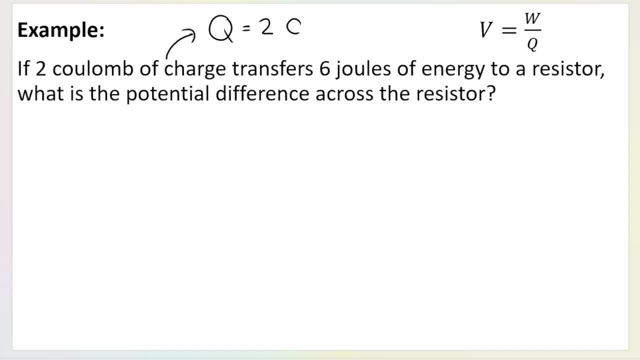 transfers six joules of energy- remember, energy and work is the same thing. so work or energy doesn't matter- is equal to six joules. what is the potential difference across the resistor? so we're looking for v. so we're looking for v. we've got q, we've got e or w, so we use the following formula: 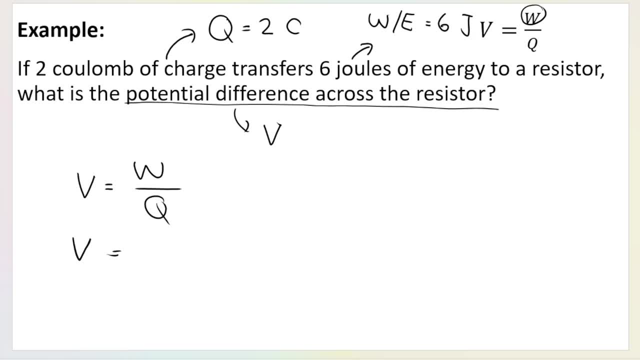 we're looking for potential difference. the energy transferred or work done is six joules and q is the charge. it's two coulombs. so that means that the voltage or the potential difference is three volts. another thing that i just want to show you is that the energy transferred or work done is: 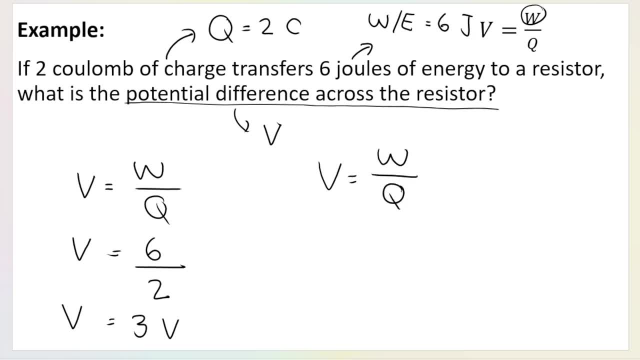 b or di times t. i think lets say that this is v. so if you would just like to measure the energy transfer or work done, it is a IN side chilled here and the voltage has to be b all at the same time. Δ peak and V peak is the voltage transferred, is Vp, Mp and the polar impulse cost contract gives us 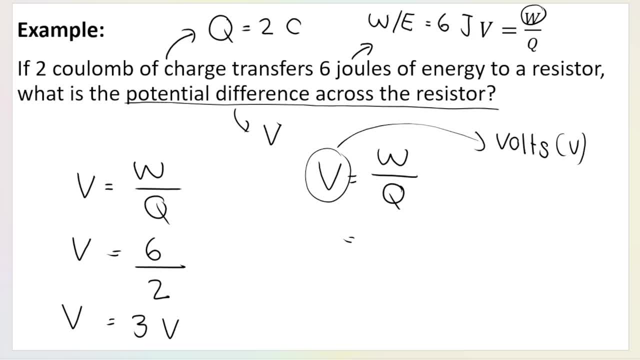 a mantra, A maus: P, A, only phi. this is our total away. we are going to divide that with theta between pB, Vp and beta. and now- now you will understand that, because that's because i just don't have Bernieian deles- we just told you that this is the direction, that we are going to be going in that direction when we will move to 3.5. 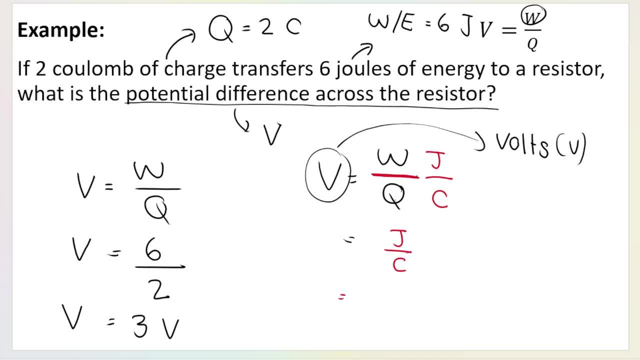 commentしま by charge. if you take charge to the top of the fraction, remember this has got an exponent of one- if we bring that to the top, it's joules per coulomb, so volts, the unit volts, is the same as the unit joules per coulomb. just a little side note because you can get asked that in a 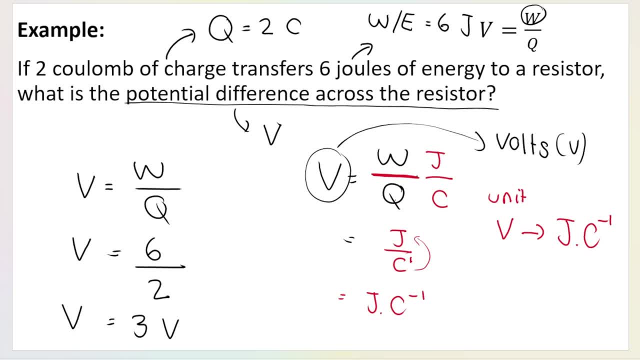 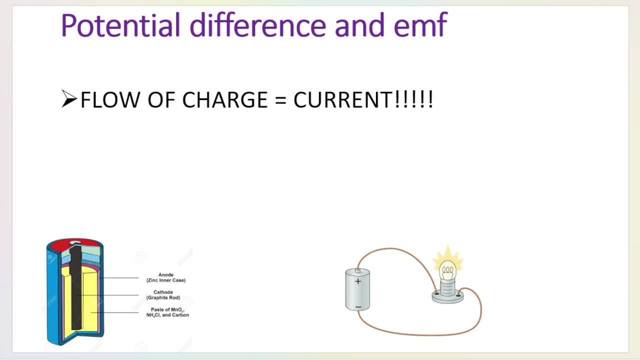 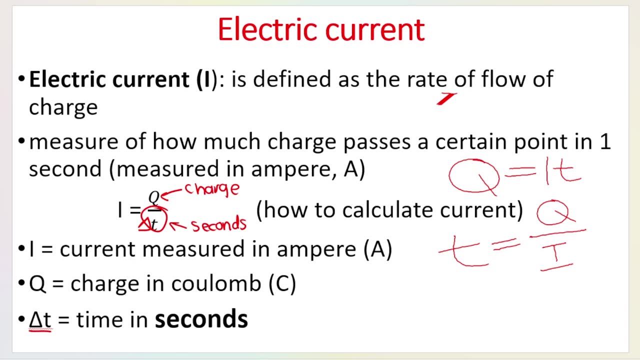 multiple choice question. so that's how we would make use of that formula. remember, let's speak about current, our next formula. so the flow of charge is current. we know current flows through circuits. as soon as the switch is closed, current flows. and here's a little bit of a summary slide. 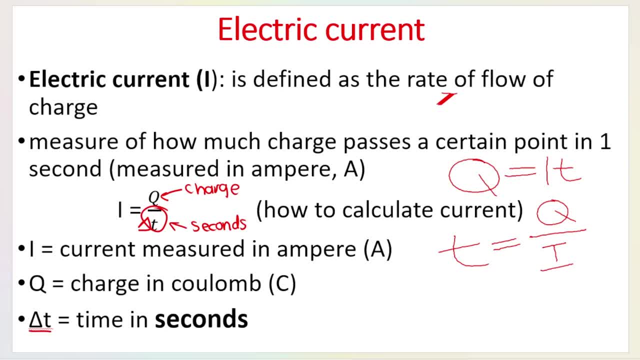 for current. so there's the definition: current is defined as the rate of flow of charge, and something that i need you to know for physics in general and chemistry, is that when you see rates, when you see the word rates, i want you to think of dividing by time, dividing by. 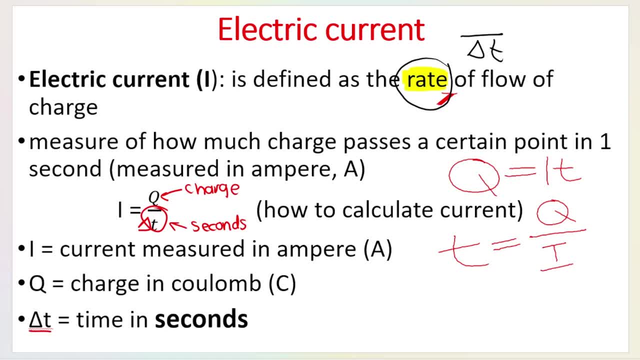 time. current is defined as the rate of flow of charge, so it's charge divided by time. that is current and that's where this formula comes from. look at our formula: current. so current is i. current is defined as the rate rate means dividing by time. see we, dividing by time. 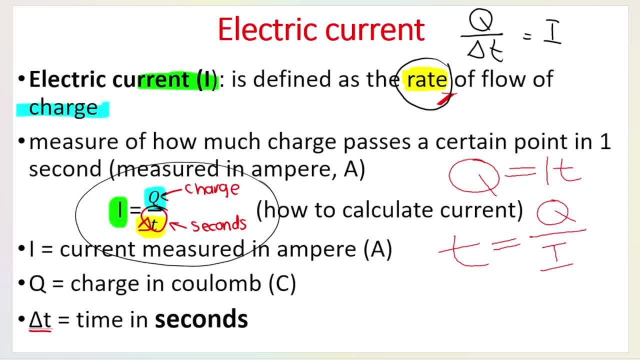 the rate of flow of charge. so charge divided by time. there we go, and, just like we did with the previous situation, we know that the unit for current is amperes, so, for example, three amperes. however, if you take a look at the formula, so current, let's do. 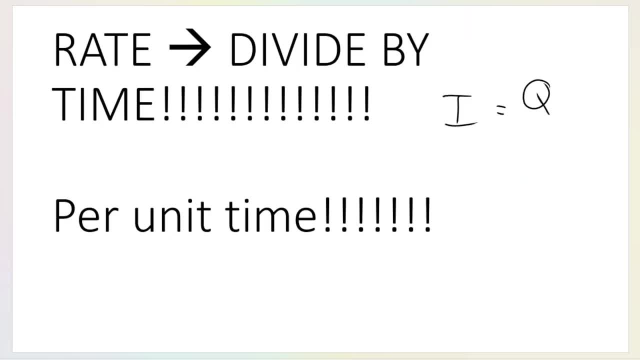 it on the side quickly. current is the rate of flow of charge, so it's charge divided by time. what is my unit for charge, coulombs? what is my unit for time, seconds? so it could also be represented like that, but i'm going to show you how to do that in just a second, so i'm going to 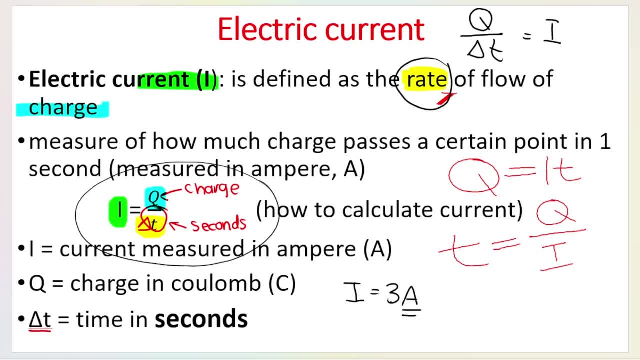 show you how to do that in just a second. so i'm going to- which is a very rare way to represent the unit. we represent it as amperes, but just be aware that they can ask you questions like that, so a type of question that you can get asked to. 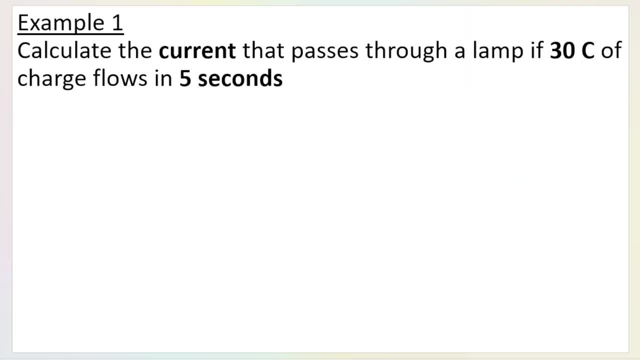 use this formula would look like this: calculate the current. so we're looking for i that passes through a lamp. so a lamp is like my resistor if the tc the t coulombs. okay, that is my charge, the t coulombs, so charge is the t coulombs. current is what i'm going to do, so i'm going to 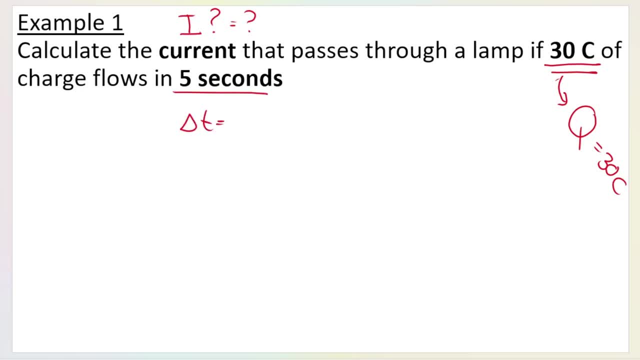 calculate the current. so i'm going to calculate the current. so i'm going to calculate the current looking for- and five seconds is my time. my change in time is five seconds, so the formula that i use is: current is equal to charge divided by time, rate of flow of charge, the t divided by five. 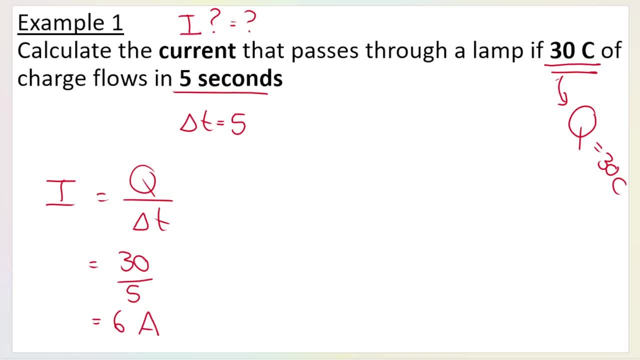 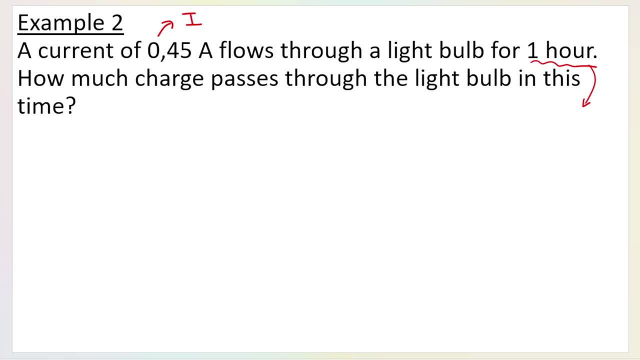 which is six amperes. that is exactly how we use that formula. take a look at a different type of question that we can get asked a current of 0.45 amperes. so they're giving me- i flows through a for one hour. this is obviously time, but time is given in hours here. it must be given in seconds. 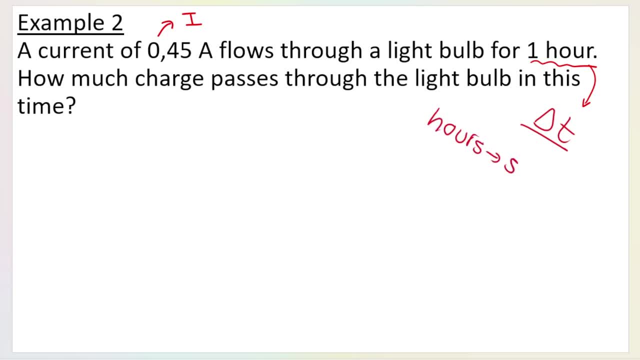 how do we convert hours to seconds? i hope you know that you need to go from hours to minutes, which is time 60, and then minutes to seconds, which is time 60 again. so to go from hours to seconds you times by 3600. okay, they want charge, so once again, you write your formula. 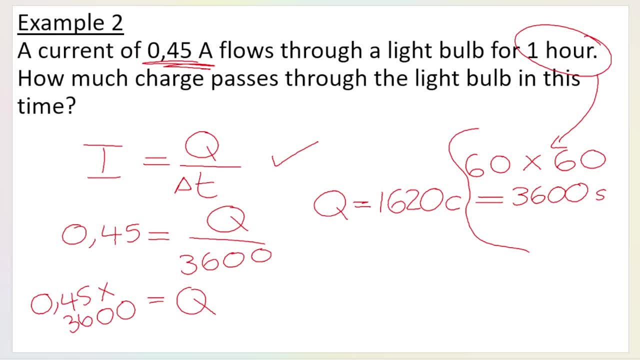 you substitute in your value. so current is 0.45. that was given time is 3600, because it was one times 60 times 60 or 1 times 3600. that's how i got it from hours to seconds and then you say 0.45. 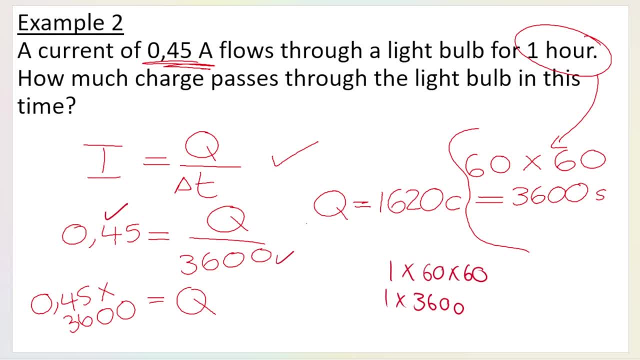 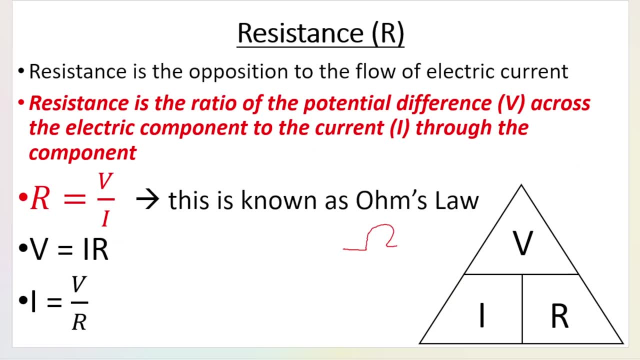 times 3600, and there's my answer with my unit. the last formula that we need to speak about is this formula over here, and this is known as ohm's law. okay, ohm's law is something that you touch on in a lot more detail. 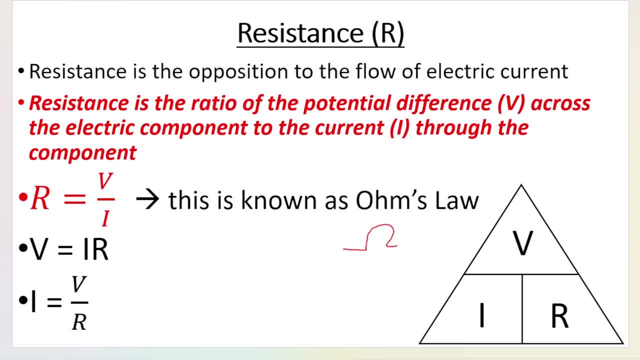 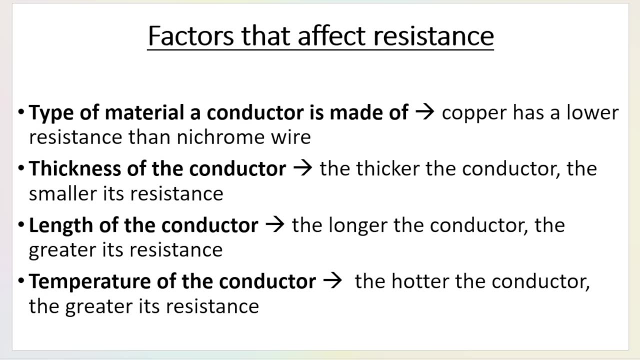 in grade 11, but for now i just want you to be familiar with the formula for ohm's law, which looks like this. you can also see it in a triangle over here. another thing that you can be asked in grade 10 is to understand the factors that affect resistance, and these are the factors that affect. 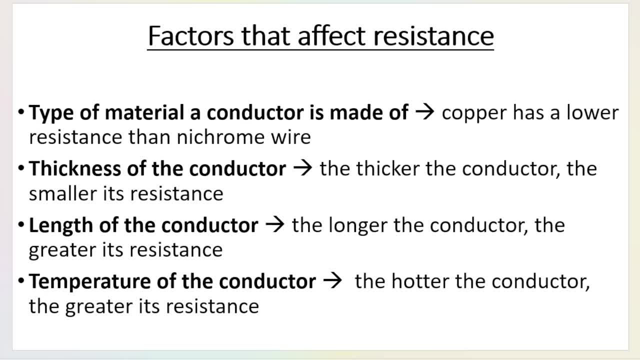 resistance. i will go through this in a separate video. you can learn this off by heart because it can pop up in your exam, and i want to quickly show you how these things are related in the relationship. this is the formula that you need to be familiar with. 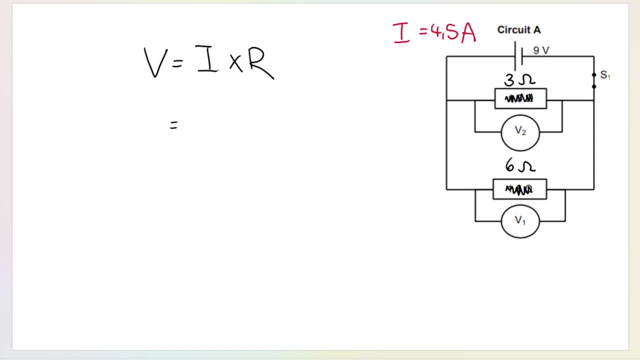 and i just want to discuss something that i hope is obvious: the total current. so i'm going to say the total current in this circuit is 4.5 amperes, which means that 4.5 the total current will flow through here. as soon as we get to a split in the circuit, the current will split and the current will 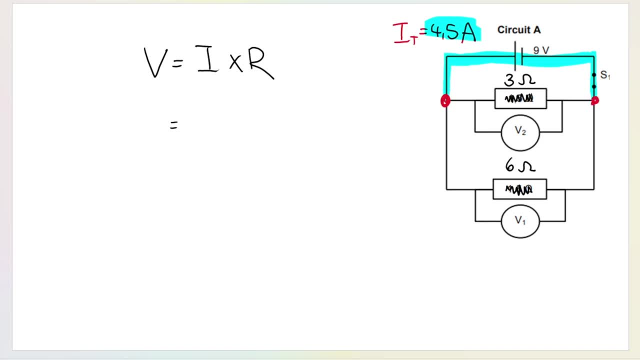 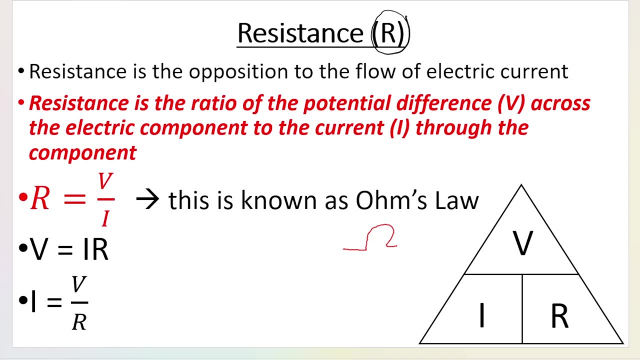 split. now one thing that i do want to ask you is remember: resistance is the opposition to the flow of current and i hope you understand that. that means if you have a high resistance, it's difficult for current to flow. so think about high resistance- difficult for you to get through high resistance. 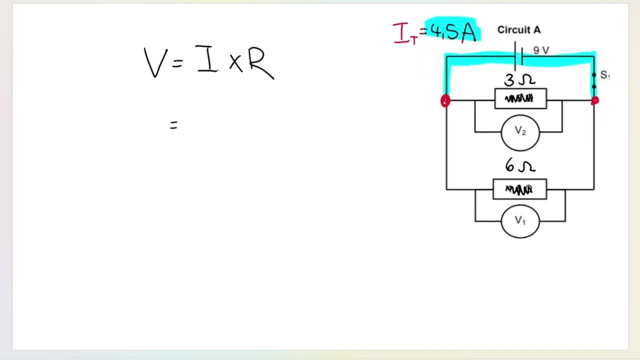 okay, so if i have two resistors, i have two resistors connected in parallel, a six ohm here and a three ohm over here. the six ohm has a bigger resistance. i'm going to write you a bigger resistance and what that means is it's more difficult to flow through this resistor. 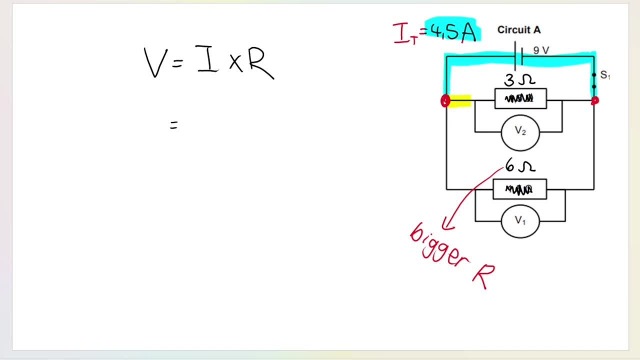 so remember, the total current will flow where you see blue. then the current will split. some of the current will go through the three ohm. the rest of the current will go through the six ohm. they split, but the split is not equal. the reason they don't split is because they don't have a 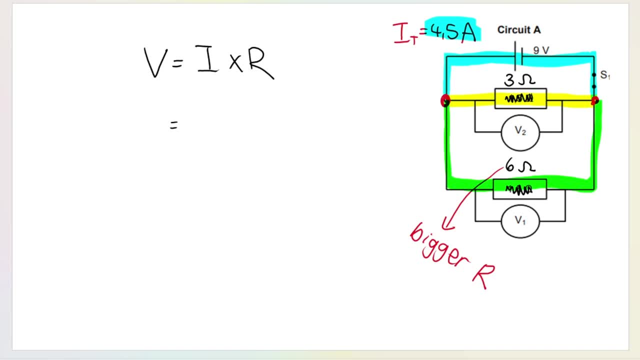 split evenly is because the resistors are different. remember, six ohms has a bigger resistance, which means it's more difficult for current to flow. so what that means is because it's more difficult for current to flow through the six ohms, there will be less current traveling through the six. 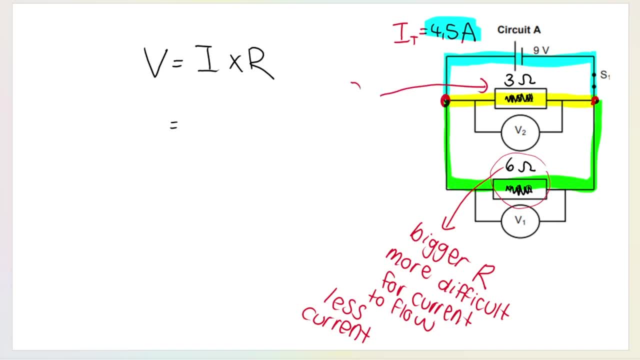 ohm resistor. for the three ohm resistor it's a smaller resistance which means more current. i hope that makes sense. if you have a smaller resistance so you're not really resisting, it's easy to flow if you are current. imagine you're a current. you see three. you're like, oh, that's not bad, three ohms, easy to. 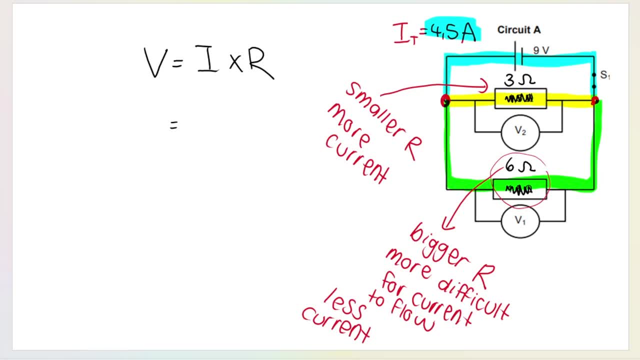 flow through there, more current will go through the yellow branch. when the current sees the six ohms, they think, oh goodness, that's a very big resistance. it's very difficult to flow through the six ohm because it's bigger, so i'm going to avoid going through there. so less current will. 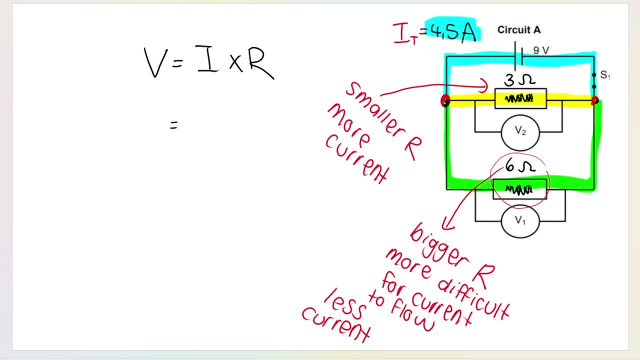 go through there okay. and i want you to always also realize that if you have a smaller resistance, make it physical and you want to becuase the actual constant is as well, it's even more powerful. but make you also realize that the signal energy functions on the state is bigger as well. 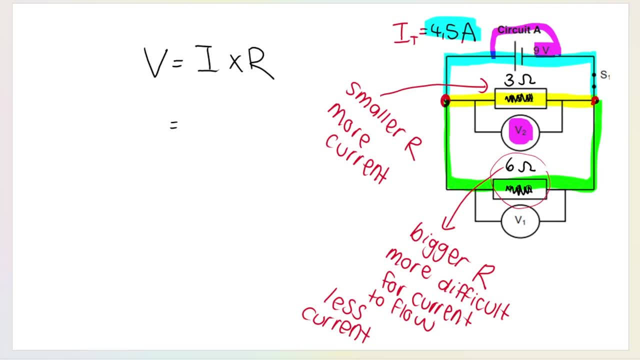 so remember we said the voltage across the battery is nine volts, which means the voltage across the three ohms is nine volts and the voltage across the six ohms is nine volts. so what that means is the voltage is the same, same voltage, constant voltage, and because that's 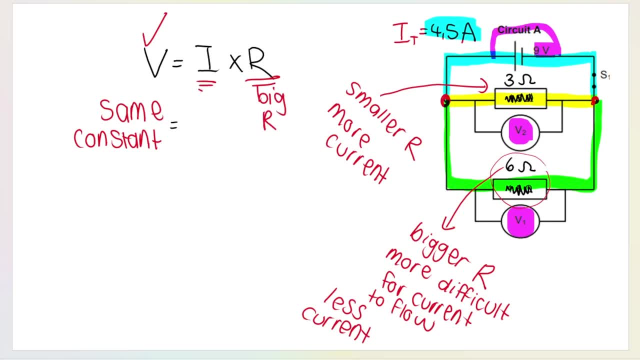 the case. if i have a big resistor, I'm going to have a small current. So just remember that the relationship between current and resistance is called inversely proportional. okay, And inversely proportional relationships, that is true. So current and resistance are inversely proportional. 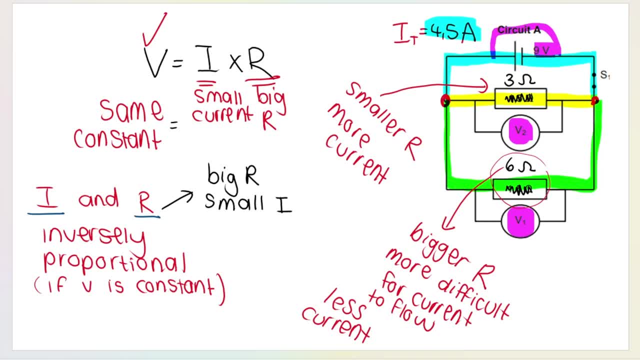 If voltage is constant, which it is because they're in parallel in this case, that means that if you have a big resistance, you have a small current. If you have a small resistance, you have a big current, And that is one thing that you absolutely need to know in grade 10.. 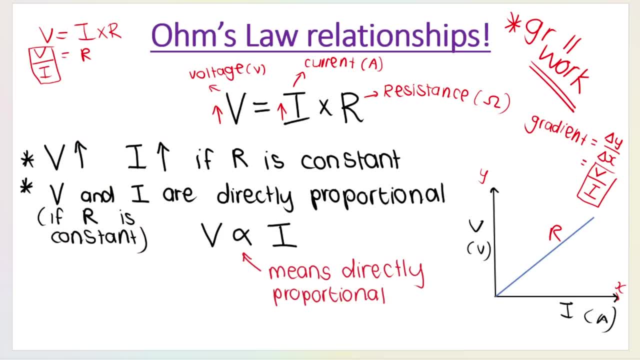 We go into this in more detail in grade 11.. You can look at these slides so long if you are interested. So there's a slide, there's a slide, And I do mention that it is more grade 11 work, but I do want you to understand this concept if you're in grade 10.. 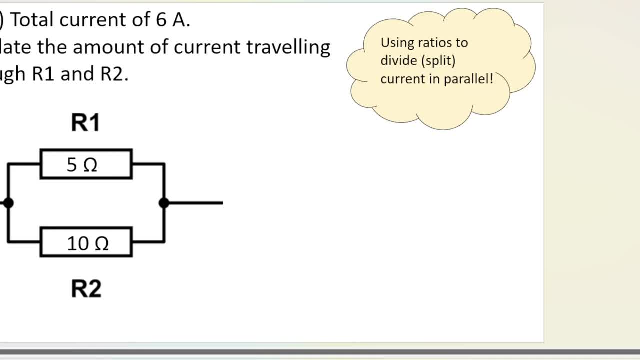 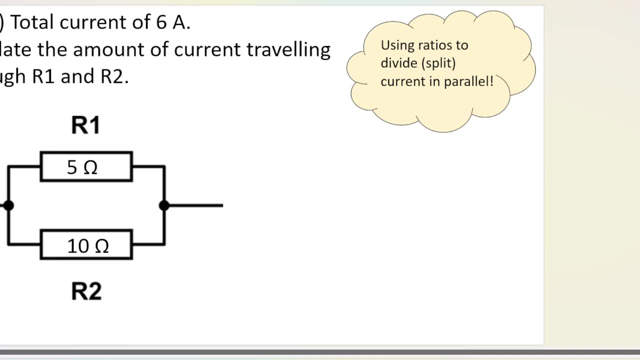 You do need to understand that And, based off of that concept, I'm going to show you how we split currents when resistors are in parallel. So I actually want to start off with a basic example, which is one that I showed you already earlier in this video. 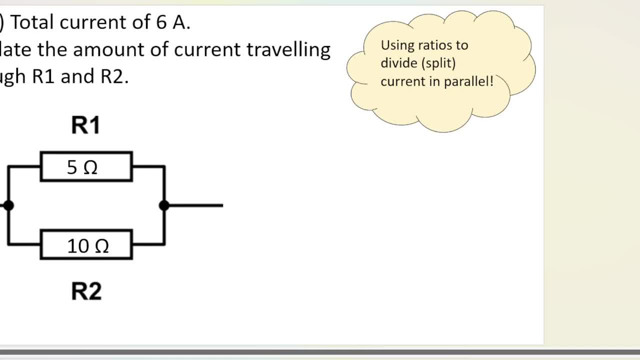 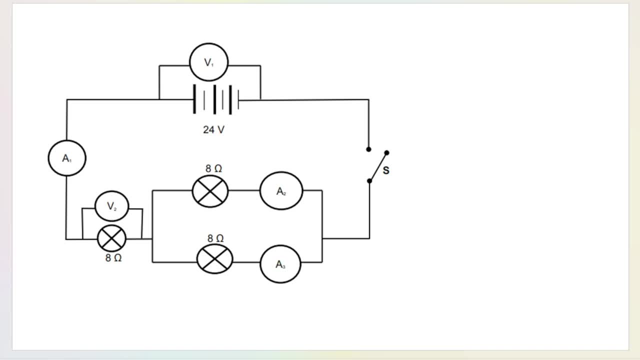 And it looks like this. Remember it was this example. okay, So I'm going to make up values for this, just to make it a bit easier, Let's pretend. Let's pretend that the total current flowing through the circuit is four amperes. 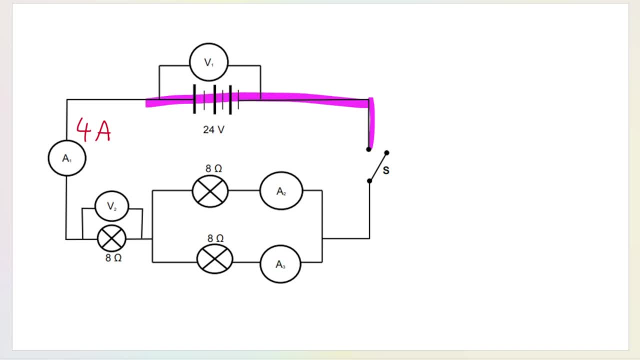 And remember what that means is total current. If that's four amperes, it will flow everywhere where I'm highlighting it in purple or pinkish color. So four amperes will flow through all of that. As soon as it reaches this point it's going to split. 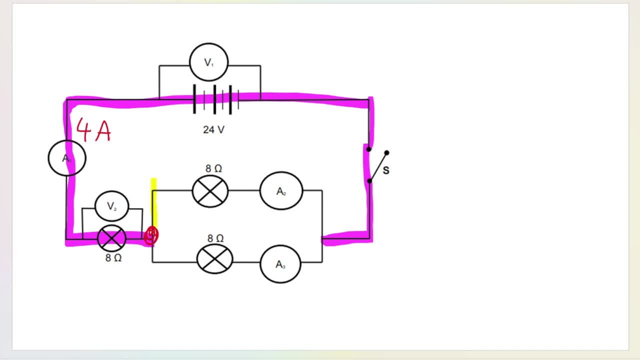 That means some of the currents will go through the top branch. The rest of the currents will go through the bottom branch, This one over here Right Now. how does the current split Right? In this case it is super, super easy, because the yellow branch 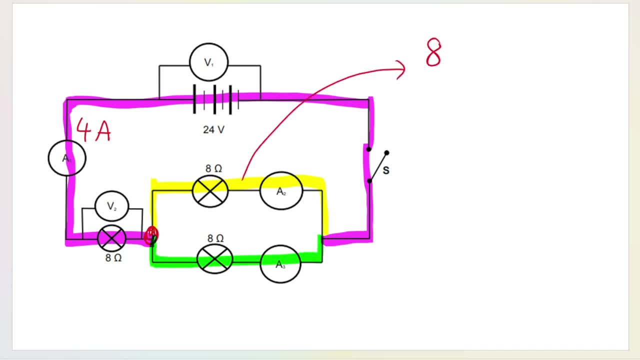 Do you see the yellow branch, The top branch, has a resistance of eight ohms. See, it just has that resistor, eight ohms. and the green branch has a resistor of eight ohms. It means that the resistances is the same. because the resistances is the same. 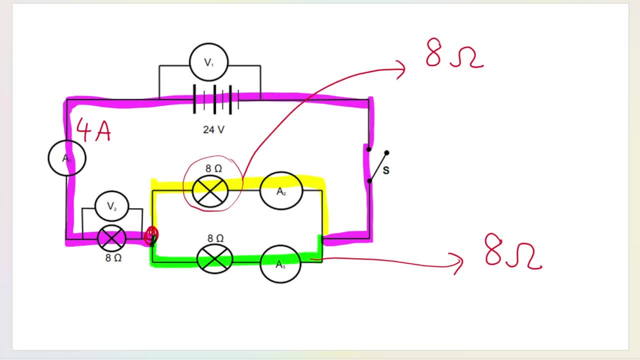 The current split will be the same, which means that the four amperes will split equally. What that means is two amperes Of current will go through the yellow branch and two amperes of current will go through the green branch. 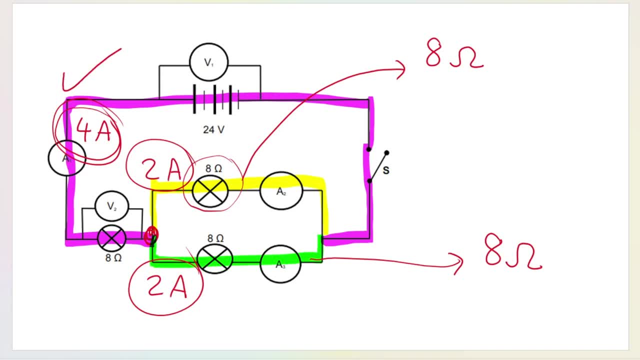 Two plus two is four- easy stuff. So the only reason that the current splits equally is because the resistance of the top branch is equal to the resistance of the bottom branch, And that is exactly what I wrote here for you, So you can take that down as a note if that helps you remember it. 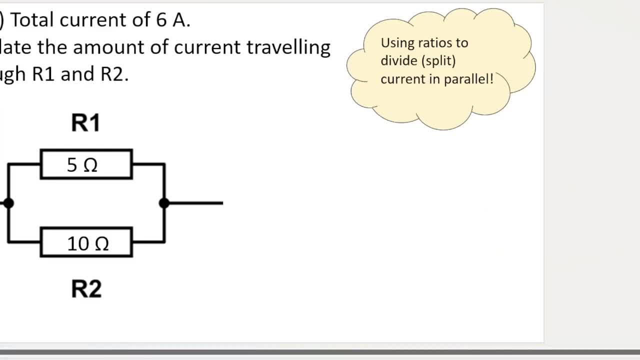 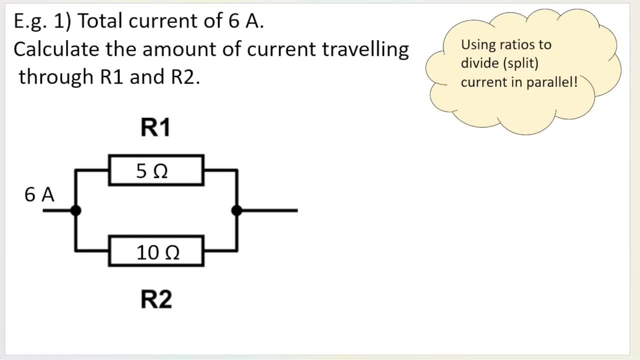 However, in this example over here, I hope that you can see That the two resistors in parallel, so they're not the same. What I've shown you on the screen over here- I hope this doesn't confuse anyone- is a snapshot of a circuit. 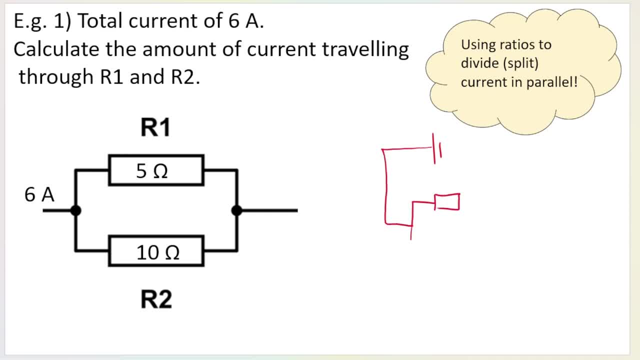 So imagine it's like a little piece of a circuit like this. So I've basically just chopped off the piece of the circuit. So the total current is six amperes and it flows through the circuit like that. So six amperes is the total current. 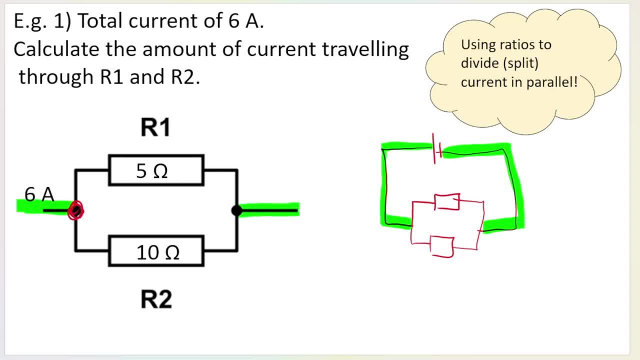 And the total current continues there And once it reaches here, the current splits. So it's just basically. what I've done is I've taken a snapshot of a circuit, The parallel resistors. that's all I've done. so don't get confused. 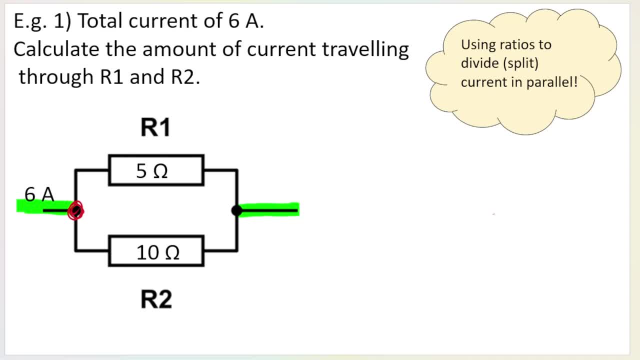 So total current is six amperes. it flows and then it stops. Some of the current will flow through the top branch, Some of the current will flow through the bottom branch, but it's not going to be three amperes and three amperes. 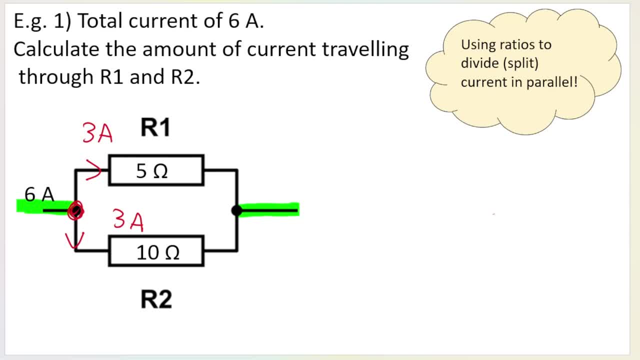 I know three plus three is six, But Are these resistors the same? No, this is five ohms and that's ten ohms. So you should know from what we've discussed which resistor should get more current. Remember, the smaller the resistance, the bigger the current. 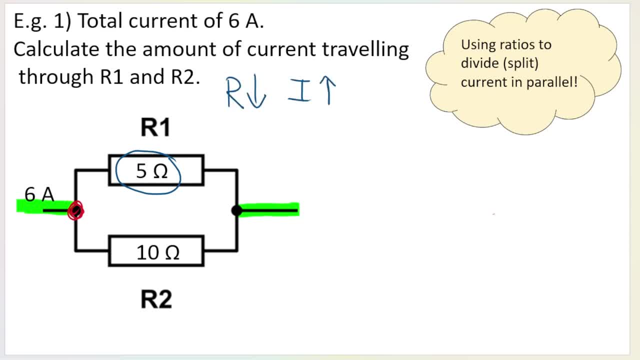 So if R is very small, current is going to be big. So because five ohms is smaller than ten ohms, five ohms will get more current. OK, small resistance, big current. And What do you notice about the ratio of these resistances? 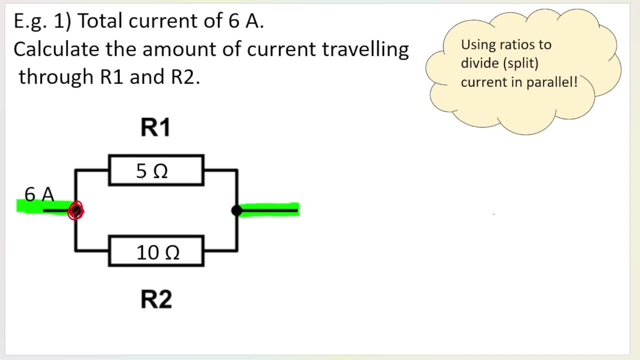 It's a one to two ratio. I'll show you that in a second. But what I mean is this: this resistor is double the size of R1. Which means that R1 should get double the current of R2.. OK, because the resistance is half, the current should be double. 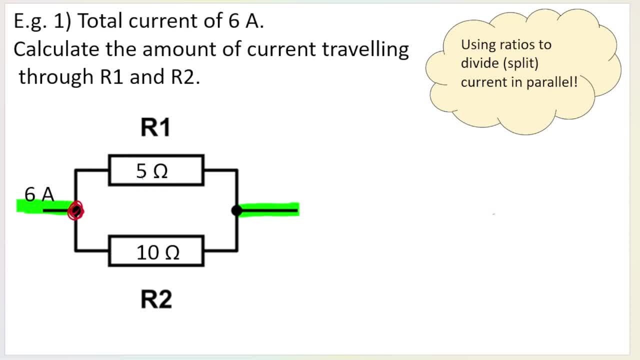 They do the opposite. Remember they inversely proportional. I'm going to show you an easy way to do this. even if it is a little bit confusing, Doing this method will always work. So how we split current is as follows: We've got R1, R2.. 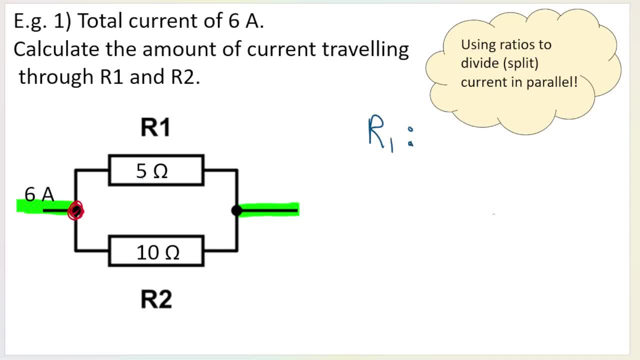 I want you to write down those resistors as a ratio: R1, R2.. Then what I want you to do is I want you to write down the ratio of resistance. So R1 is five ohms, R2 is ten ohms. 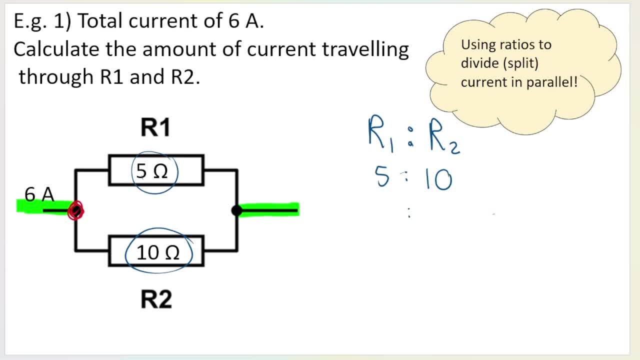 I want you to simplify that ratio. So five goes into itself once Five goes into ten. twice Five to ten is the same as one to two. Divide both sides of the ratio by five. This, what we've just written down, this is the ratio of resistance. 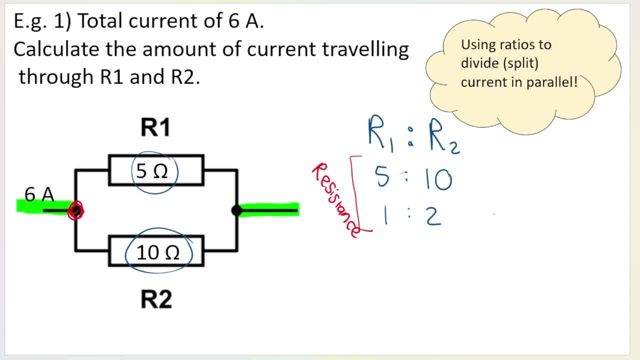 Now, what did we just learn about resistance and current? They do opposite things. So the smaller the resistance, the bigger the current. So what I want you to do- and you will always do this when you are splitting currents- is you take the ratio of resistances and you flip it. 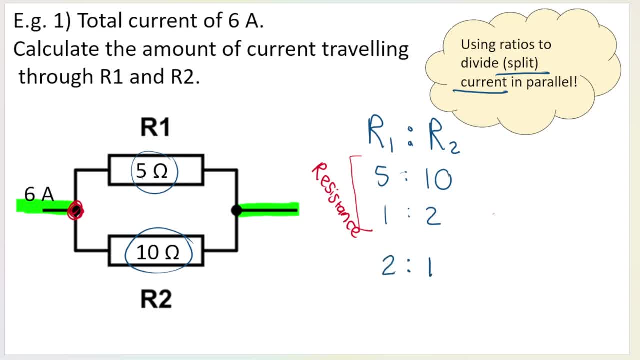 So one to two, you must write two to one. That is what I now call the ratio of currents. If that's confusing why we do it, just keep reminding yourself of the relationship. Small resistor: R1 is small, So one is smaller than two. 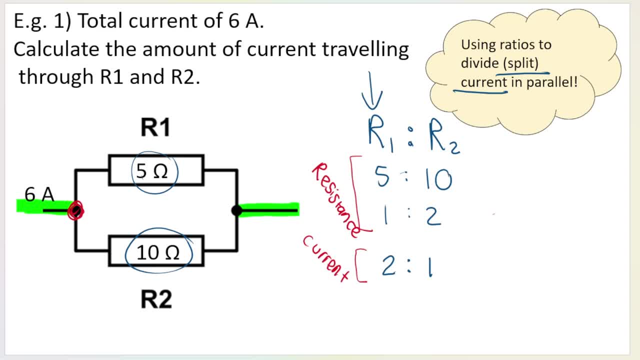 Big current two is bigger than one. Okay, So just flip it. Just flip the ratio. So you write the ratio of resistances five to ten, simplify it and flip it. Now what we're going to do is something that we did in grade nine: math. 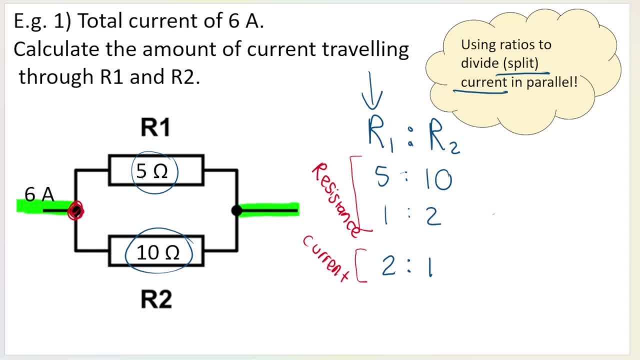 in grade eight math, where we split something into a ratio. So you may have learned splitting into a ratio differently, in different ways, but what you do is you add the parts of the ratio together. So two plus one is three. Two plus one is three. 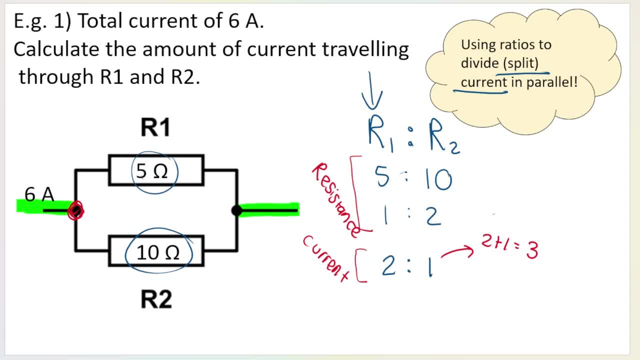 And what we now do is we say, okay, if I want to work out the current going through R1. So I'm going to write that at the bottom here: Current in R1. What I do is I take the part of the ratio that corresponds to R1. 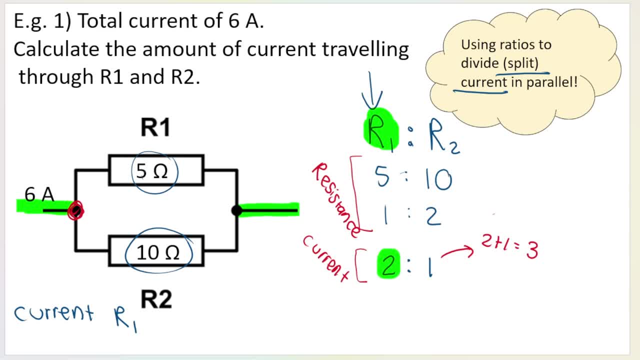 So you follow R1 all the way down to the bottom. It's two, So you go two over three. Why over three? Because the total parts of the ratio is three. So two corresponds to R1, and we're looking for the current in R1,. 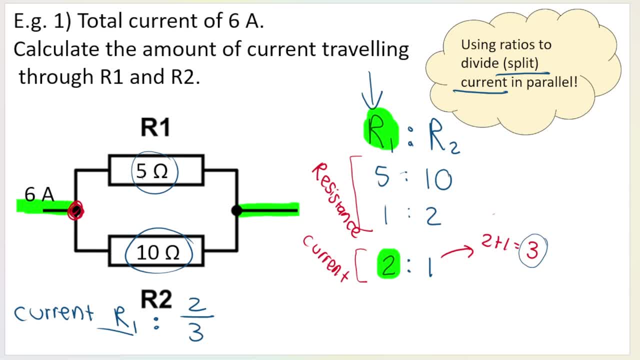 and we're looking for the current in R1.. So we're looking for the current in R2.. So we're looking for the current in R1,, two over three, because the total parts is three times by the total current, which is six amperes. 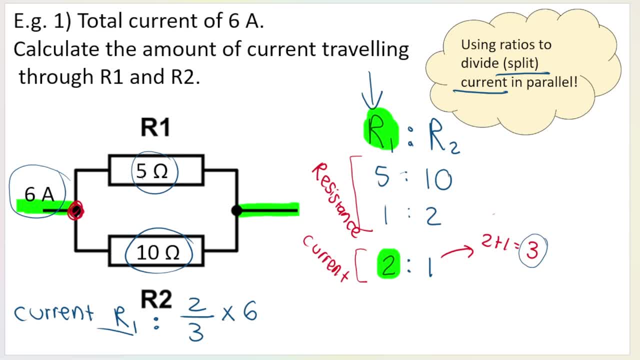 i gave it to you over there. so basically, what i'm saying is the one ohm sorry, r1, the five ohm resistor. r1 gets two thirds of the total current, and two thirds of the total current is four amperes. okay, we can do the same thing, but for the current through r2. so what you do is so that 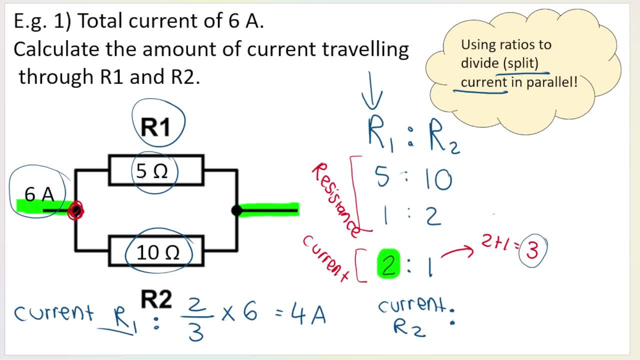 was current through r1 should actually use a different color here, so let's use: current through. r1 is yellow. okay, current through r1 is yellow. you go with, you follow r1 all the way to the bottom two. so current through r1 is two over three. it's always over the total parts. 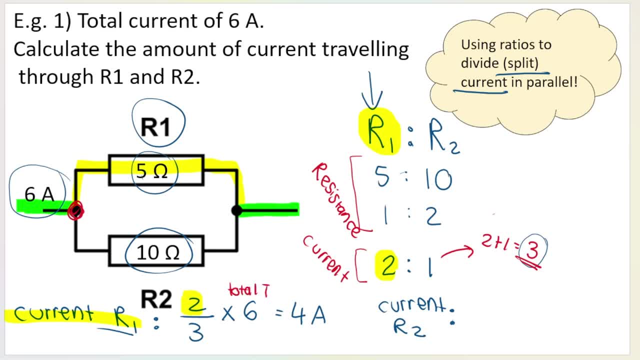 times the total current is two over three. it's always over the total. damn things we did in the current. so you always times the total current. let's do it for r2, let's see if it makes sense. so we take r2. remember r2 will get the rest of the current. you follow it all the way down to. 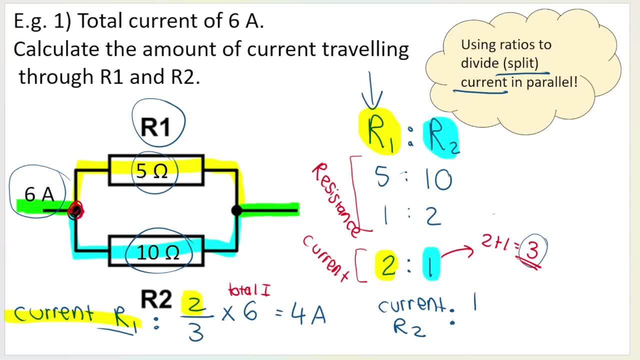 the bottom it's one. so we go one over three times the total current times six and that gets you two amperes. one over three times six. so this is two over three times six, this is one over three times six. so in both cases you multiply by total current. in both cases you dividing by the total, 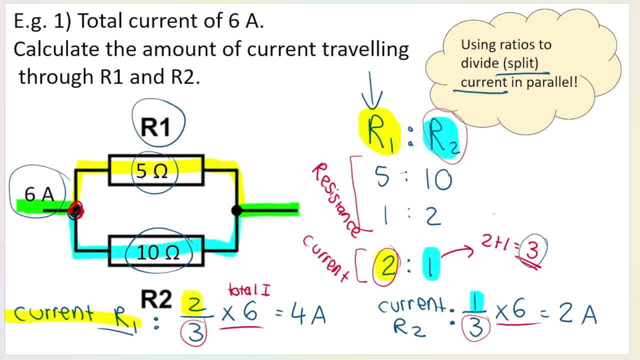 part of the ratio. for r1 you use two, for r2 you use one and it makes sense, think about it carefully. so the total current is six amperes. r1 gets four amperes, r2 gets two amperes. and we did say 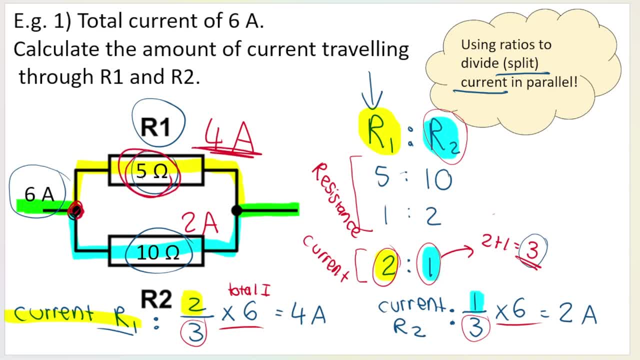 that the smaller resistor will get the bigger current. the bigger resistor gets the smaller current currents. we also said R1 is half the size of R2.. 5 is half the size of 10.. And because R1 is half the size in resistance, it gets double. the current 4 amperes is double 2 amperes. I really, really.